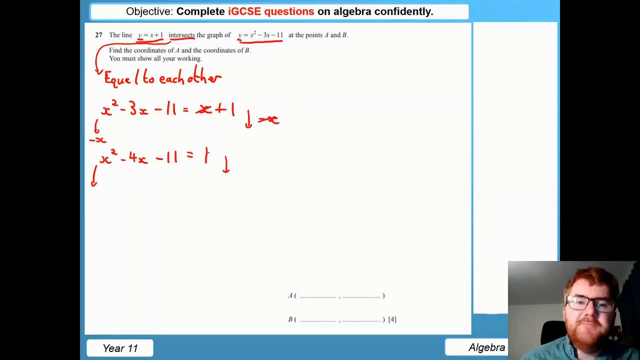 step, if you so wish, but just to go through what's going on here And now. if I want to make the right hand side zero, I want to minus 1 from both sides. x squared stays the same. minus 4x stays the same. minus 11 minus 1, be careful with this. that is minus 12. 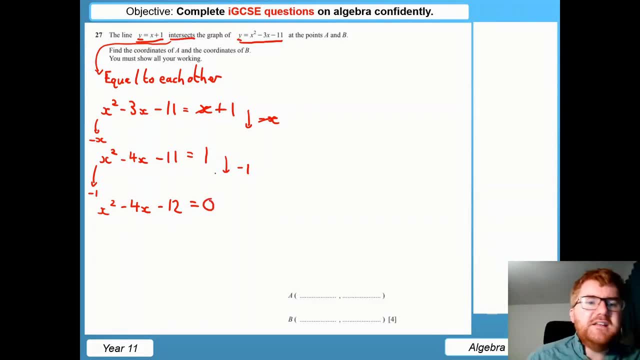 equal to zero. At this point, we need to do some factorizing. okay, This is the easiest way to solve these equations, So I'm going to set up my brackets and remember the two key rules. I'm going to highlight this. so if we do this a bit later on, you're going 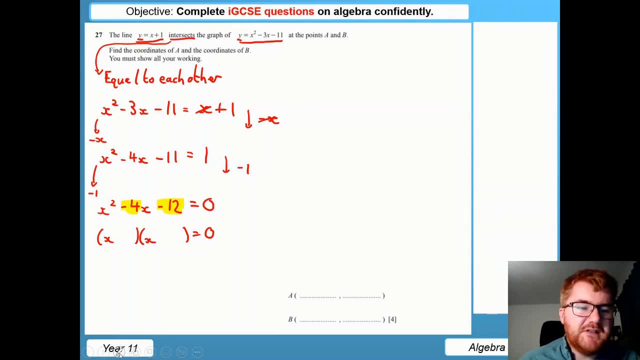 to see this in action. So I want two numbers that multiply to give me minus 12, but I want two numbers that add also to minus 4.. Now one way you can do this is actually just write out combinations that multiply to give you. 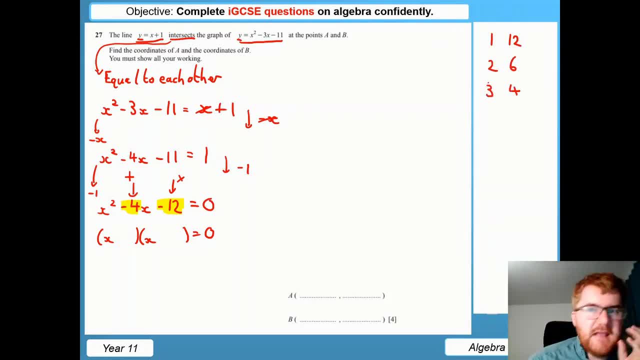 12, and then see what works from here. And if we have a quick look at this, if I put a minus here in front of the 6,, well, minus 6 times 2 is minus 12, good stuff. and then 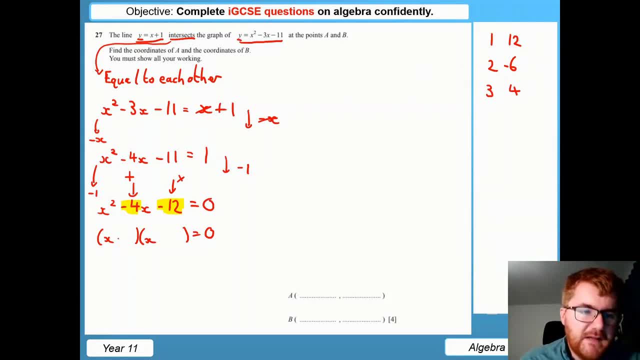 minus 6 plus 2 is equal to minus 4.. So I've found the numbers. they go into my brackets. This is the easiest way of solving. Try not to go straight to the quadratic formula. do at least think about trying to factorize. Now we have two brackets here and they are: 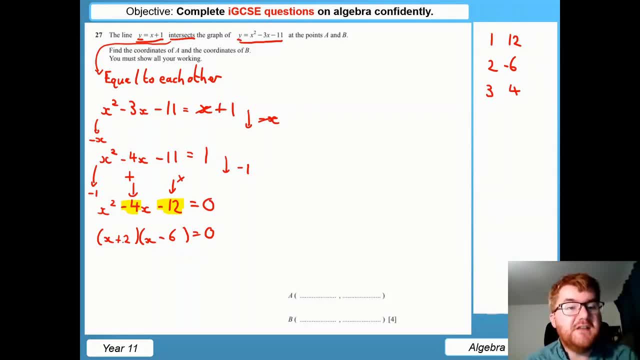 equal to zero. So you have two things multiplied to give you zero. that means either one bracket is zero, so x plus 2 is zero, which then means that x is equal to minus 2, or- and this is the alternative- the other bracket, x minus 6, is equal to zero. 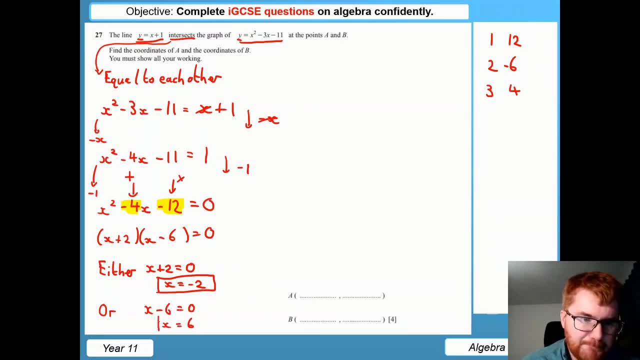 In which case then x is equal to 6.. Now, at this point- do not celebrate, you do not have all four marks- at this point, I'm going to put minus 2 and 6 as my x coordinates, because we now need to find the y coordinates. Now, whenever you have a linear function, so y. 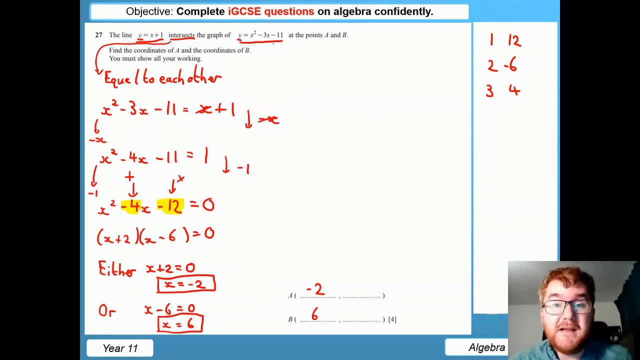 equals x plus 1, you should really substitute into that. it makes your life easier. So when x is equal to minus 2, y is equal to minus 2 plus 1, and that's equal to minus 1.. When x is equal to 6, y is equal to 6 plus 1, which then gives me the y coordinates for. 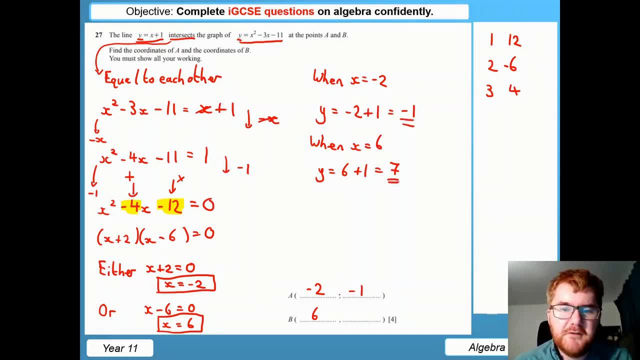 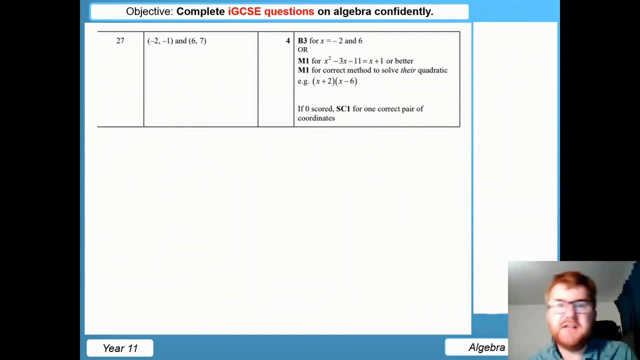 each point. So our final answer here is minus 2, minus 1, and 6, 7.. Again, you can look at the mark scheme and see how we work our way through that. You get three marks. even if you don't substitute in for y, you'll still get three marks out of four on this question. 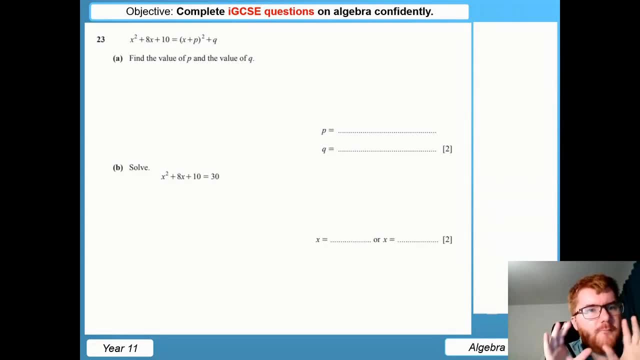 Alright, let's look at now quadratics in a slightly different way. This is quite an interesting question from 0580.. So you're given, x squared plus 8x plus 10 is equal to this expression. Now you might know this as completing the square, which always drives horror into the 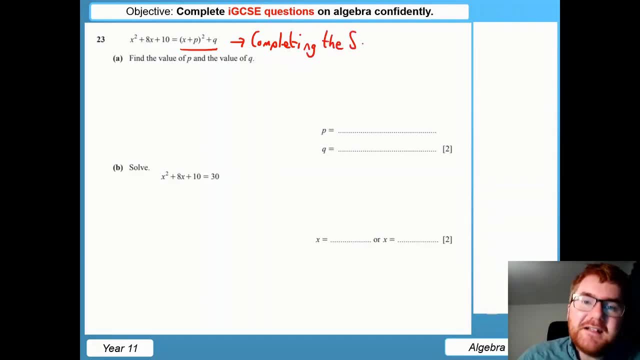 hearts of students completing the square. If you want practice on this, then do check out the video above. I go through this in more detail Now. I'm going to take a slightly different approach to this and then simply expand out the right hand side. Now remember. 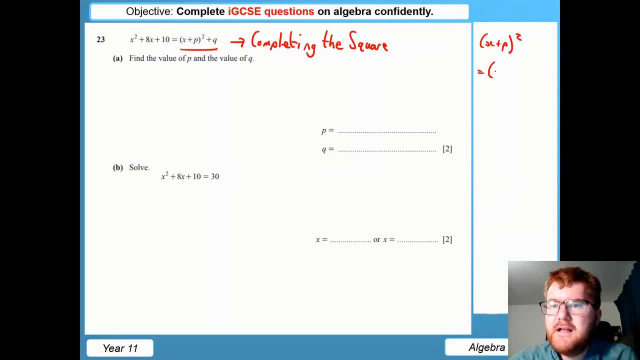 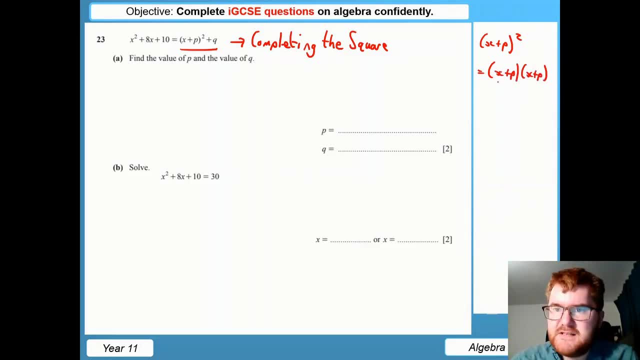 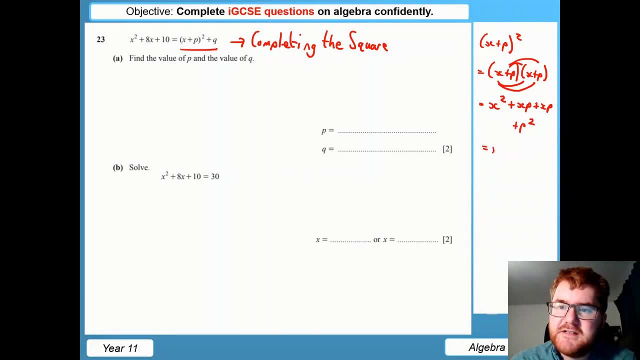 times p is p squared. If we collect up like terms, which is always important, I have one xp, I have another xp, that's 2xp plus p squared. So what I'm going to do is copy out this equation and, instead of an x plus p, all squared, I'm going to replace it with what I just worked. 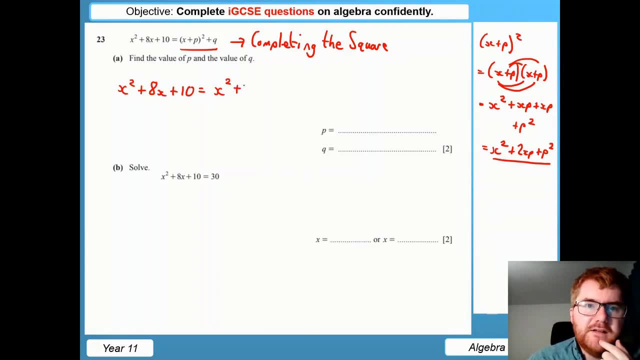 out on the right hand side. So x squared plus 2, well, let's do 2px. we'll see why. in that moment plus p squared. and don't forget, the plus q is also there too. And now what we're going to do is we're going to copy out this equation and, instead of an x plus p, 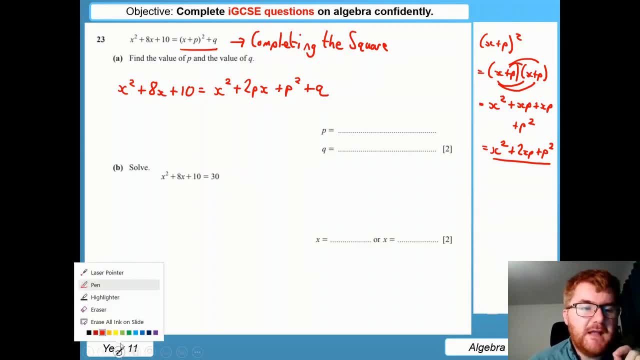 we're going to do here is something called equating coefficients. Now, what do I mean by that? Well, I look at the coefficient of x here, which is 8.. That has to be the same as the coefficient on the right-hand side, ie, these two things highlighted must be. 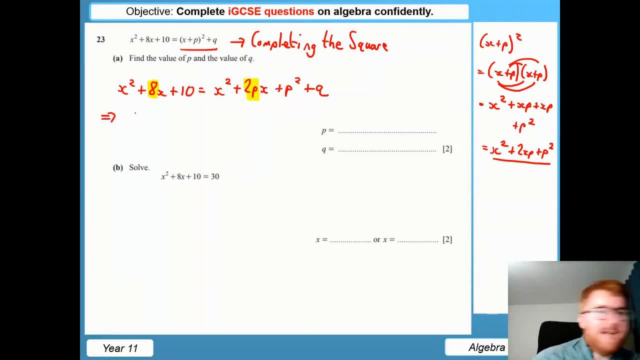 equal to each other. Notice that intersecting is always coming up, isn't it? So we get: 2p is equal to 8, and therefore p must equal, then 4.. So that's the easy one. We can pop over there and, using the same idea here, this 10 must be equal to the constant term. 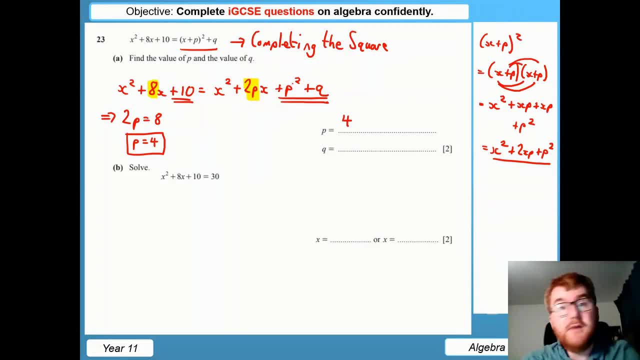 so this p squared plus q- Now we know what p squared is now, because p is 4, so 4 squared is 16.. So we get: 10 is equal to 16 plus q and therefore we can take 16 from both sides. 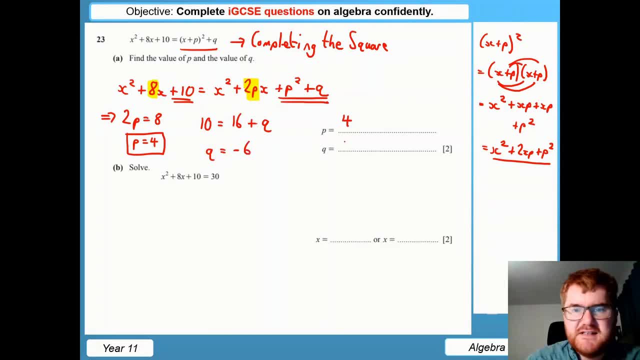 here. giving you q is equal to minus 6 for the two marks. So I've taken this approach. Again, you can take different, You can take different approaches on this kind of question, but I thought equating coefficients is so useful down the line when you do IB or A level. It's a really important skill. to see. Now, this is very typical on. this is the paper 4 question. here. They now want you to solve this equation. Well, the first thing I notice here is that the left-hand side is same as part A. So notice, I can swap over the left-hand side here with the right-hand. 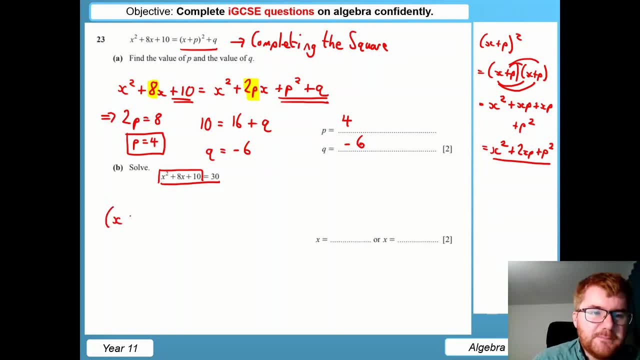 side. So what I'm going to do now is I'm going to right-hand side, So I'm going to right-hand side, So I'm going to solve this equation PCX, and what this is going to do is I'm going to take this left-hand side and I'm going to do the same thing. the 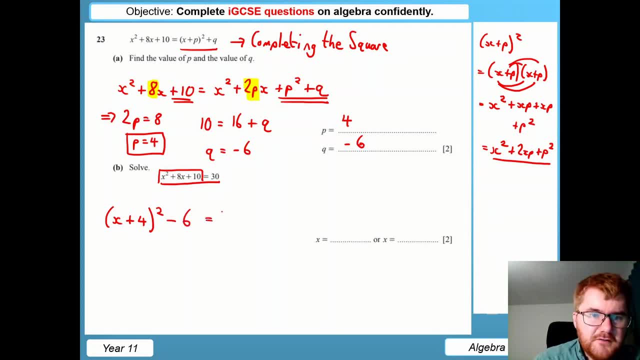 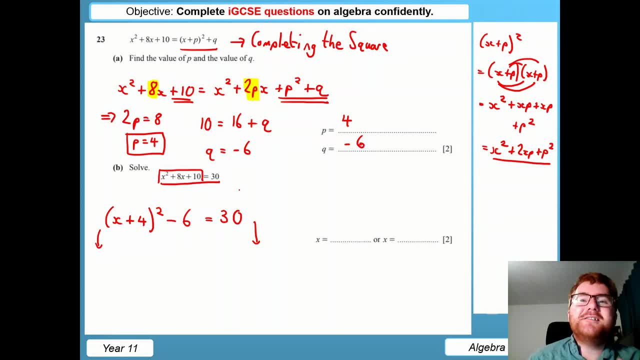 right-hand side hit 16 right here, and I'd just writeê- Because I can subtract it, so I don't have to WhatsApp- that I can just say fold up 20.. So I'll write a fold here: 6 on both sides. this cancels, leaving us with just this bracket. and then 30 plus 6 is 36. now the 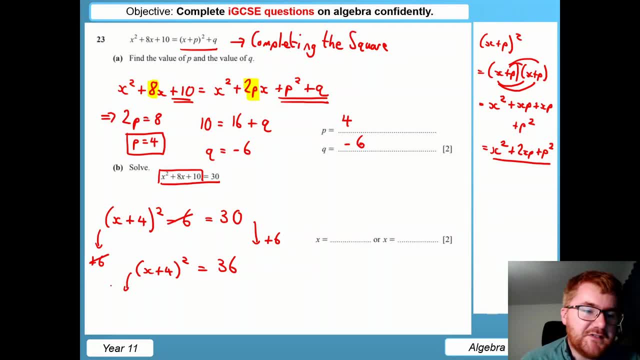 squaring is annoying me because I want to get x on its own here. so what's the opposite of squaring? well, we're going to square root both sides. this is where we have to be a bit careful, so we're going to cancel here, and that leaves us with x plus 4. and remember, the square root of 36 isn't just 6. 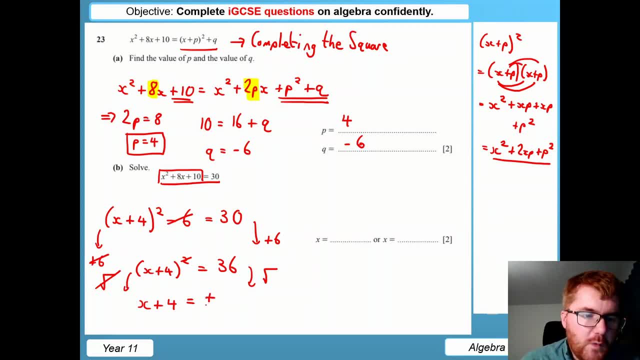 it's also minus 6 as well. so the square root of 36 is plus minus 6, because remember, minus 6 times minus 6 is also 36 as well. at this point we then just treat it like a normal equation. so we have a plus 4 here. so what's the opposite of that? well, we're going to do minus 4 on both. 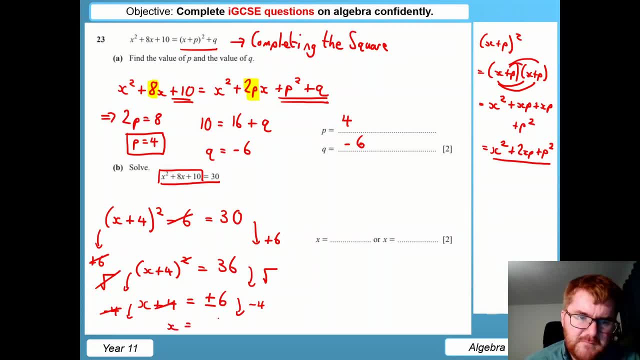 sides. this cancels, leaving us with x, and then we get plus minus 6, minus 4. now you're probably thinking: what's the opposite of that? well, we're going to do minus 4 on both sides. this cancels, leaving us with x, and then we get plus minus 6, minus 4. now you're probably thinking: what's the? 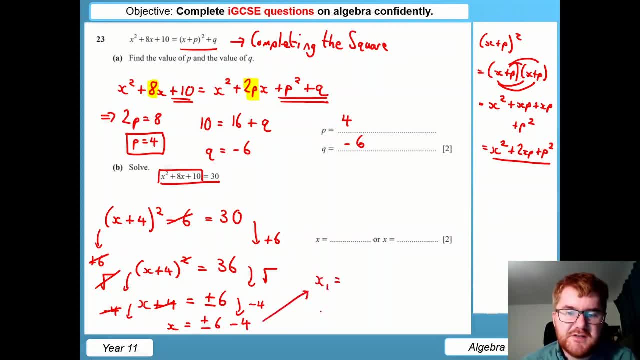 opposite of that. well, we're going to do minus 6 minus 4. now you're probably thinking: how do we work that out? well, we work it out as two different solutions. so first of all, we're going to pretend it's a positive, so we get 6 minus 4, which is equal to 2. that's our first answer. and then we 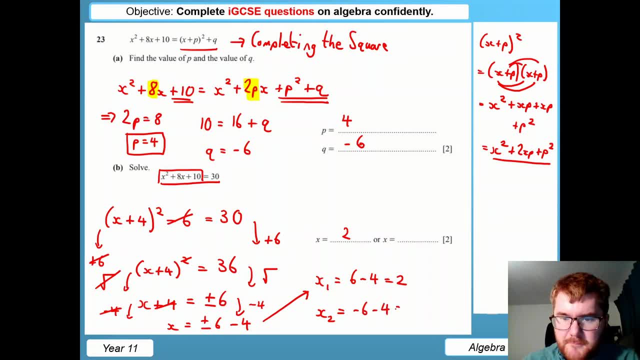 pretend it's a minus, so we get minus 6 minus 4, which you don't like negative numbers. you have a calculator, so use it, but we get minus 10 for the second mark. so I've included this question in here because it uses obviously quadratics but also different star. 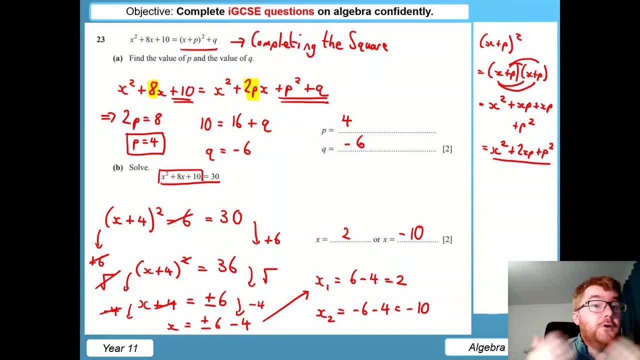 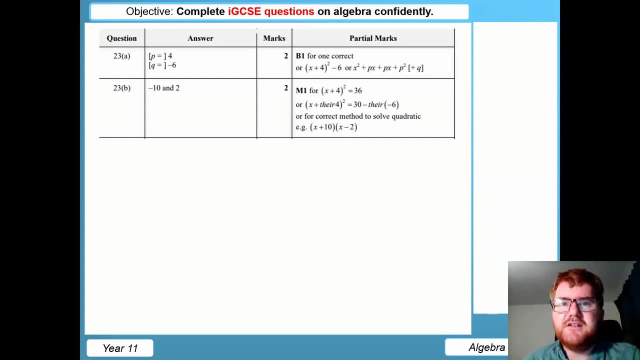 of questions, if you're aiming for those higher grades, really gives you exposure to the style of question they could give you. again, you can check through the answers and check through all the working I've done in that question. okay, and on to some worded questions. so you need to. 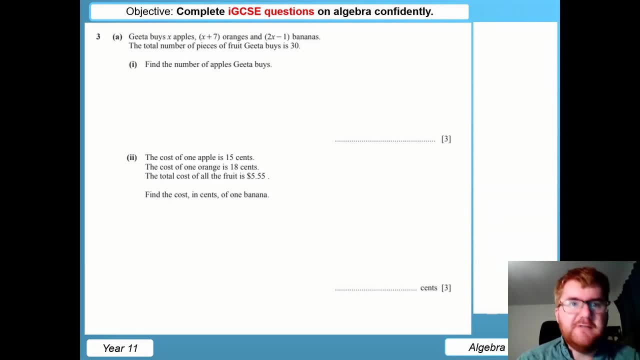 make sure you're happy with worded questions- they can pop up in a variety of different forms- and making sure you can translate that language there into equations you can solve. so let's get started. so Gita buys x apples- I'm going to underline this. so Gita buys 7 oranges and 2x minus 1 bananas. a lot of fruit there and the total number of pieces. 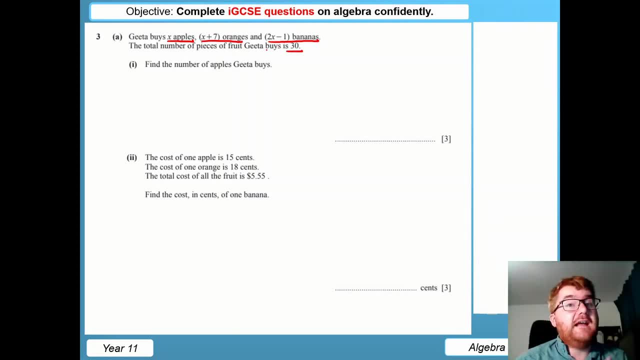 of it is 30 and from that we need to work out how many apples Gita buys. so if we take, we have x apples. if we add the amount of oranges, which is x plus 7, and then we add on the number of bananas, 2x minus. 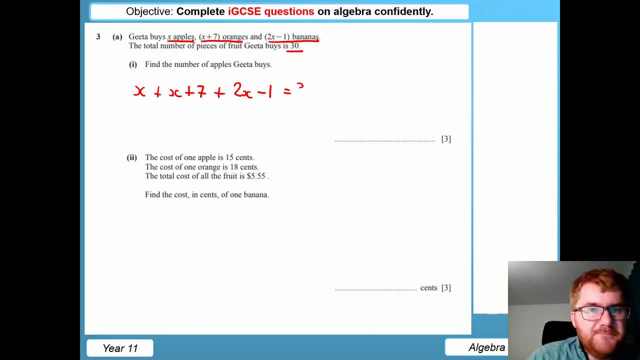 1, that needs to equal 30. so notice, by a quick translation of the question into the language we know, we can then get a problem we can solve. at this point we have 2x here, an x and an x, that's 4x. so 2x plus 1x plus 1x is 4x. 7 minus 1 is equal to plus 6 and that's equal to 30. from there we use 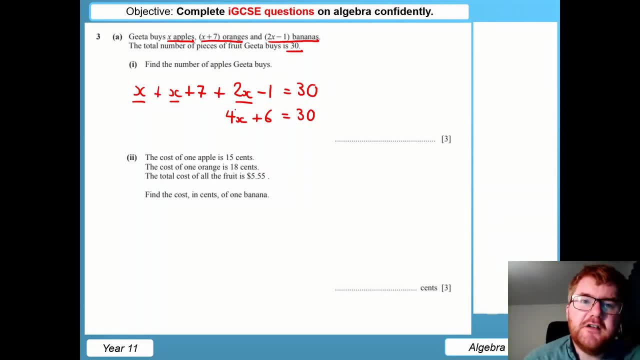 our normal equation solving methods. so you want to get x on its own. the plus 6 is annoying. what's opposite of plus 6? well, that's minus 6 on both sides. this cancels, leaving us with 4x, and then 30 minus 6 is 24. you can probably see the answer. 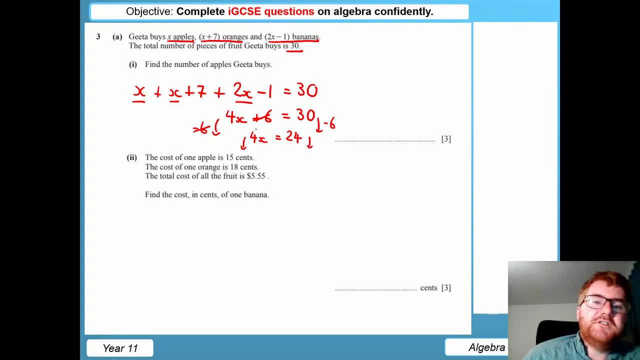 remember the method that we use here. what's the opposite of timesing by 4? that's dividing by 4 on both sides. now that cancels, leaving us with x is equal to 24 divided by 4, and that is 6. now remember, x itself actually represents the number of apples that are bought by Gita. 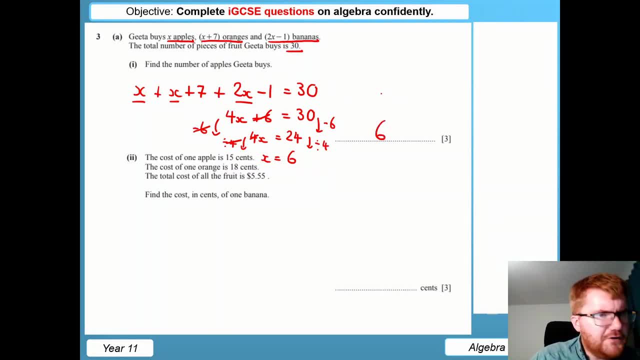 how often are problems our answer? now this felt like the more context in among people gone on by eliminating the bankrupt. you choose what works, how hard you have to change the reportable. I know you are able to move from one to more interesting example- Turkey- and I closed it down so you can have a pretty brief idea of what. 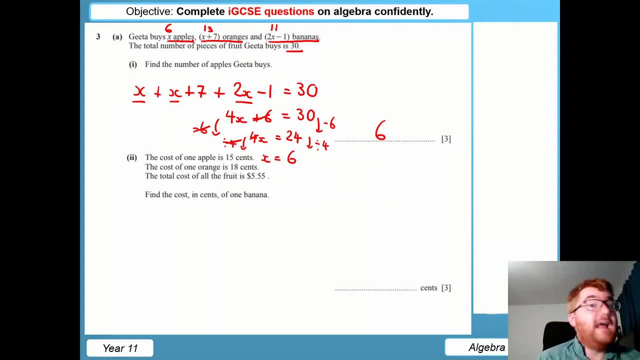 happens within 6 months and how you can operate and pay the tax which risk you not just� now. quick advice: I'm never sure, too. when people fee, you can and money us. one orange is 18 cents and the total cost is $5.55, also known as 555 cents, and we need the cost of 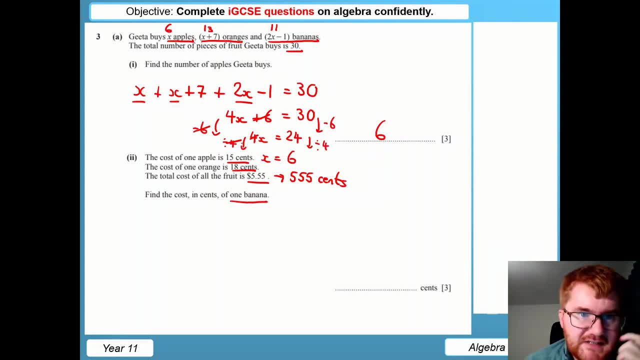 one banana. So the way I'd approach this is: well, let's work out the total cost of all the apples. well, each apple costs 15 cents and there are six of them, so we do 15 times six, then we add on the total cost of all the oranges. well, there are 13 oranges at 18 cents, so 18 times 13, and then we've 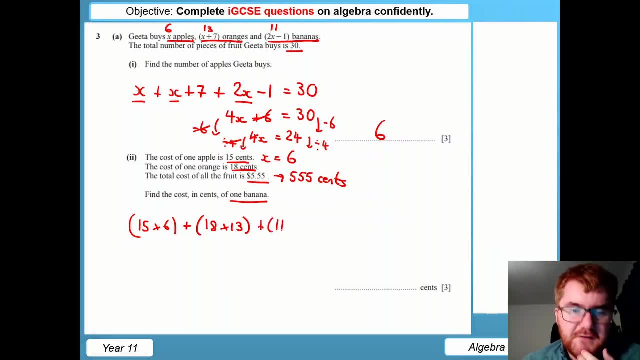 got 11 bananas, but we don't know the cost of it, so we call it 11 times b. so we call b for the cost of one banana and this is equal to 555.. So if we simplify this down here again, a lot of this you. 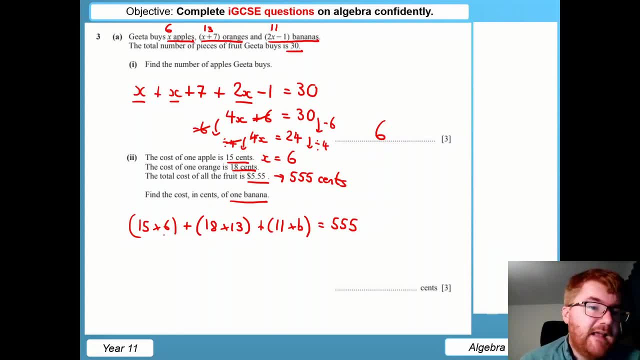 can do on your calculator, so don't feel like you have to do this manually. 15 times 6, that's going to be equal to 90, and then we're going to do 18 times 13 here. so 18 times 13 is 234, and then we've got 11 times b, which is just 11b, and then we have 555.. Notice. 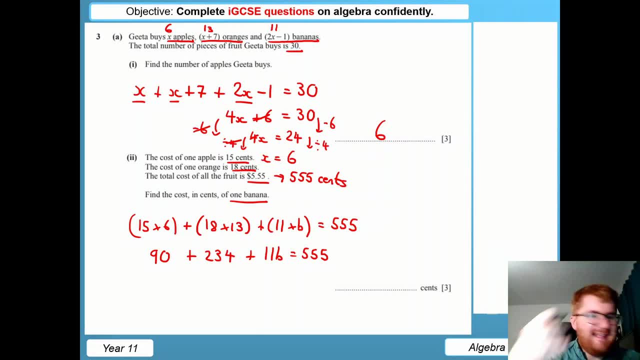 the way I've set up the equation here, once I work out b. that is my answer and I can just write it down. So if we tidy this up slightly, 234 plus 90- then use your calculator, don't be shy. so we get 11b plus 324.. Notice addition: you can. 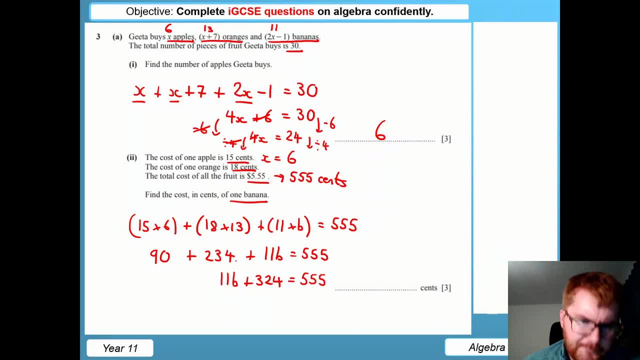 swap around is equal to 555, then we're going to do exactly the same process as above, of course, the opposite of adding 324, minusing 324 on both sides. that cancelling here, giving us 11b and 555, minusing 324 on both sides. that cancelling here, giving us 11b and 555, minusing 324 on both sides. 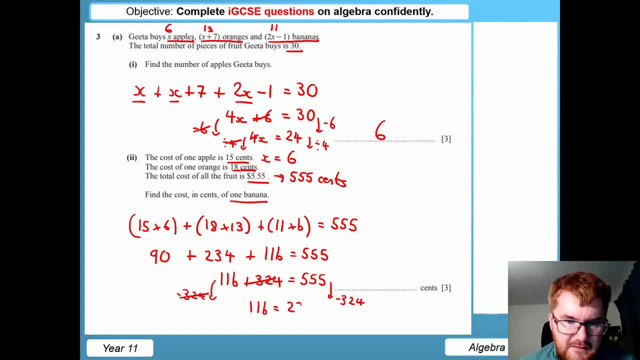 that cancelling here, giving us 11b and 555 minus 324 is 231, and then we don't like times 11b. so what's the opposite? divide by 11 on both sides, and if you get a whole number here, that is probably a. 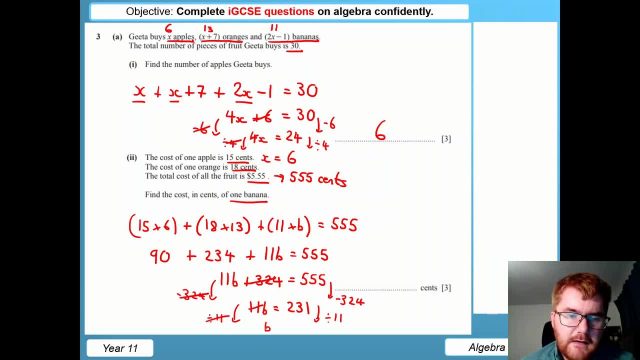 very good sign. So we get b on the left hand side and we get 21 on the right hand side. If you get a whole number, it's always always a good sign. so we're going to pop that in as our answer for three marks. 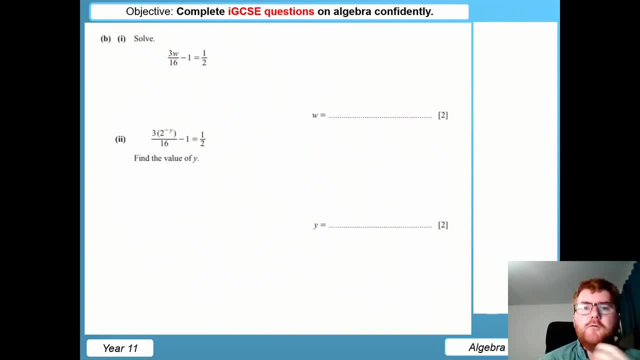 Now this question from paper four is quite involved, so be aware of that. if they put algebra into a paper four, it's going to be lots of different skills being tested. so you get lots of really good practice in this video. So here we need to solve this equation here. so 3w over 16. 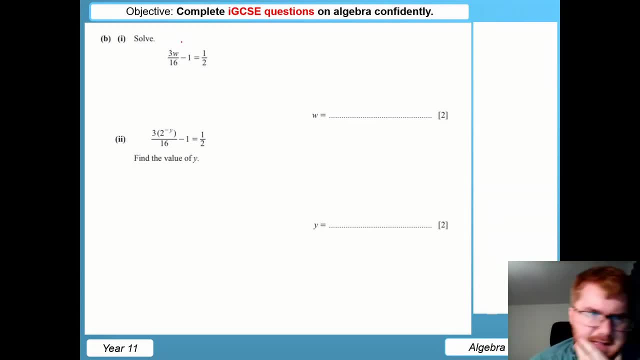 minus 1 is equal to half. So I'm going to take a mixture of approaches. in this case, I'm going to start with the minus 1 being annoying, as it often is when it's just after the variable. so the opposite of minus 1 here is plus 1.. So I'm going to take a mixture of approaches. in this case, I'm going to start with the minus 1 being annoying, as it often is when it's just after the variable. so the opposite of minus 1 here is plus 1.. So it's a little more difficult to do, but hopefully you'll work it out. 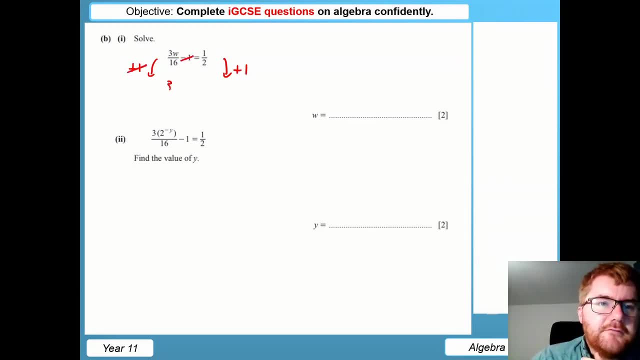 On both sides. that gives us, if we cancel here, 3w over 16 and 1 plus a half. well, that's the same as 1 and a half, or 3 over 2.. So again, there's a couple of different ways you can approach. 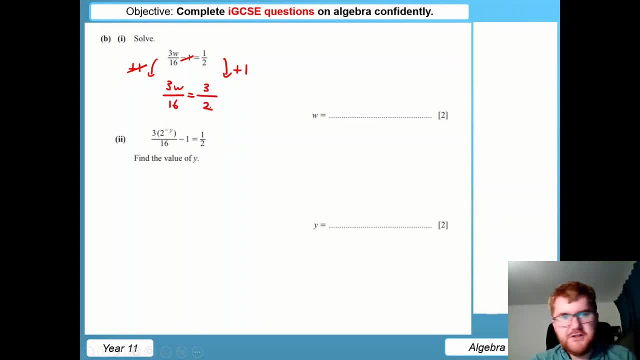 this. I'm going to write this as an improper fraction, and you're going to see why. next, When you have fraction equals fraction, you can do a process called cross multiplying. It's a very useful technique. You're going to start out with the first two simple ones, so you'll start with the 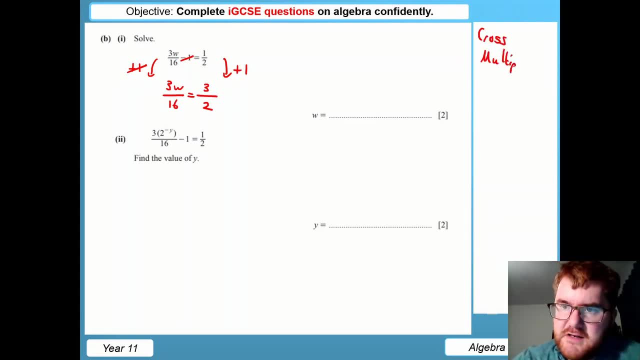 first two simple ones. You're going to start with the first two simple ones and then you'll start with the you're going to see in this video as we go through now. what do I mean by this? well, if I times this by this and this, by this, you get this cross idea. we can. 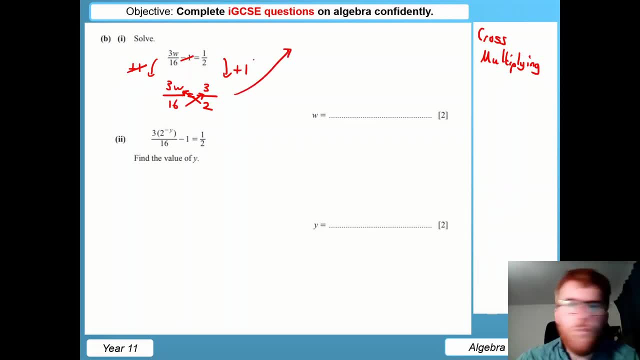 actually simplify this down to an easy equation. okay, what do I actually mean here? so 3 W times 2, that's equal to 6 W, and then 16 times 3 is equal to 48. it's a really nifty way of actually removing the fraction very, very quickly. and now. 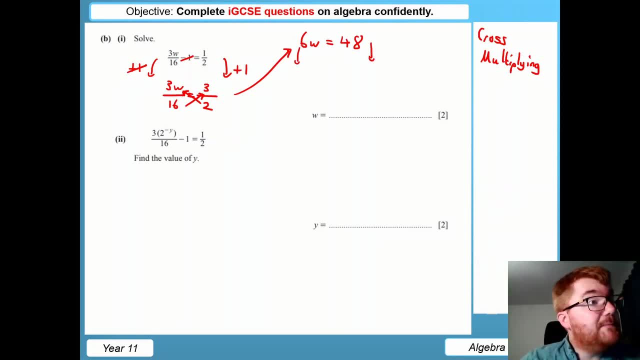 we have a nice easy process here. so what's the opposite of times in by 6? we're going to divide by 6 on both sides. that cancels giving us W. 48 divided by 6 is equal to 8. again, use that calculator if you need it now. I like this style of. 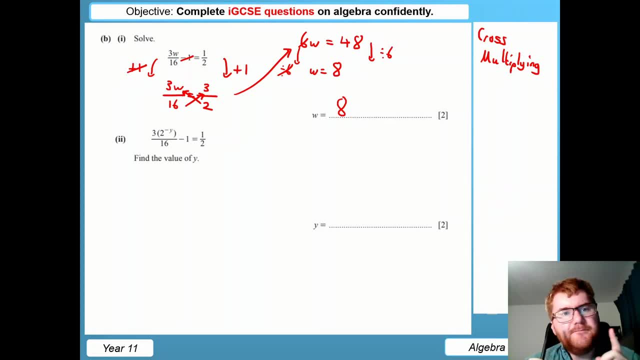 question. this a a star element of the question. I look at it and then I think to myself: well, it's almost. I think to myself: well, it's almost identical to exactly what I've just been doing. the only difference is, instead of a W, let get the highlighter out here. instead of a W here. all they've. 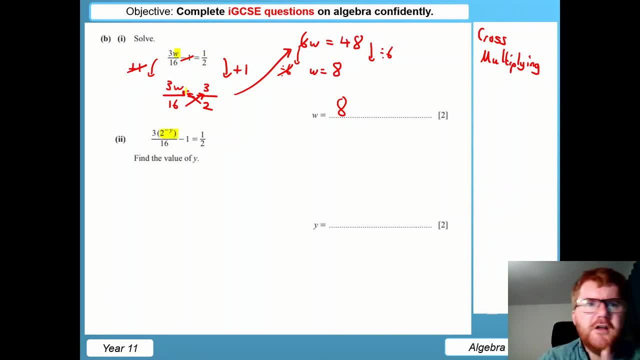 put is a 2 to the power of minus Y. well, if I know, for the first equation the W is equal to 8. in the second equation, what's highlighted here, this 2 to the power of minus Y must also be equal to 8 as well, and this saves you doing a lot. 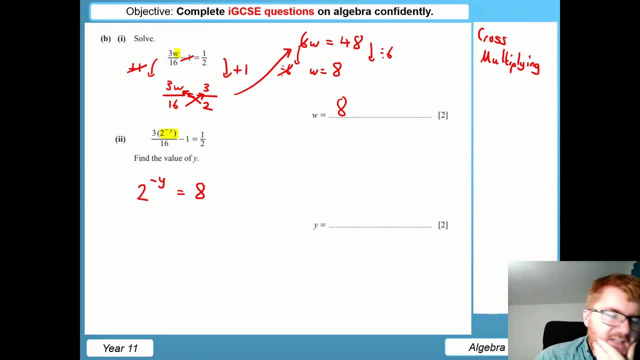 of working for a two mark question now at this point, to actually work out what Y is here, there's a couple of different approaches you can take. I'm going to try and make the right hand side of this equation look like the left hand side. so what do I mean by this? well, 2 to the 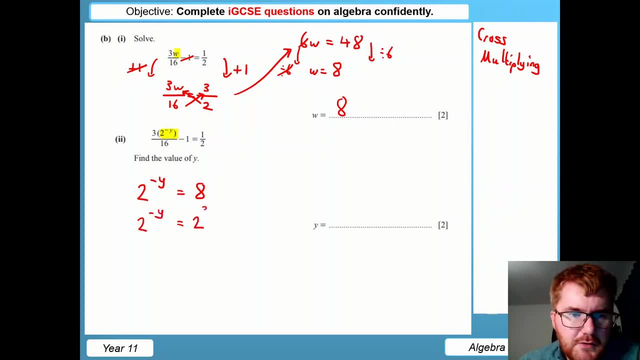 power of minus Y. what? 8 is the same as 2, canuciate. and notice, now we've got this base, the same again. I can raise both sides. this gives me then minus Y is equal to 3, and therefore Y 2 or 4.. 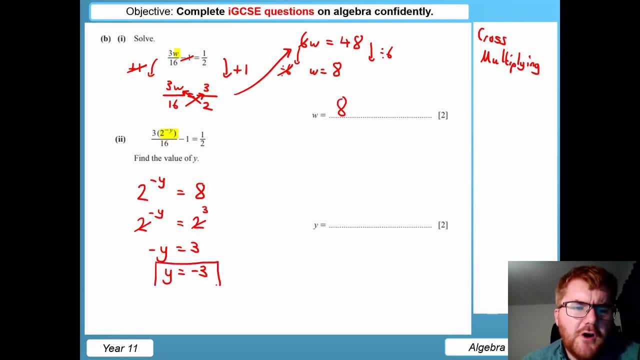 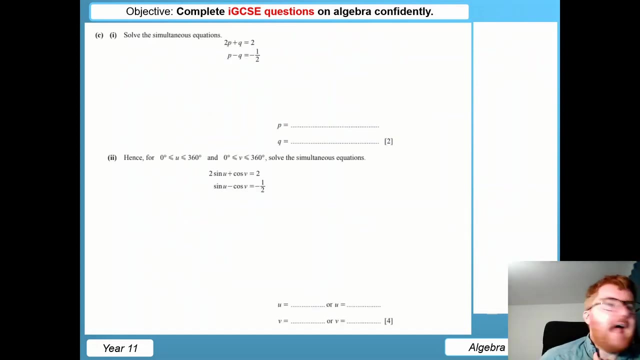 therefore, is minus 3.. To really get these top marks at IGCSE, you need to look for elegant ways to get to the answer. It's going to save you time for those really difficult mensuration, those vector, those differentiation questions right at the end of the paper. And we're not finished with this. 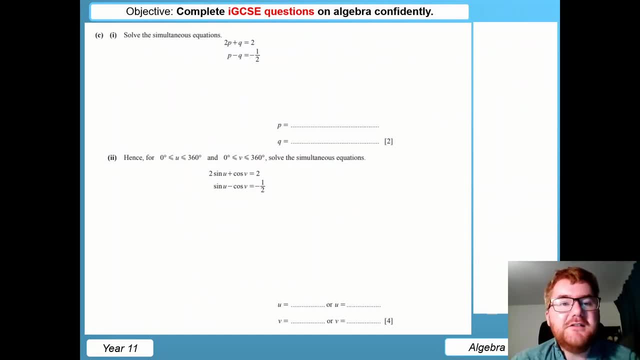 question. It keeps on going. And now we're into simultaneous equation territory, also a very important skill that I wanted to include in this video, And typically part two, where we're mixing a bit of trig in, there is a typical A star question. Now let's do the standard part here. 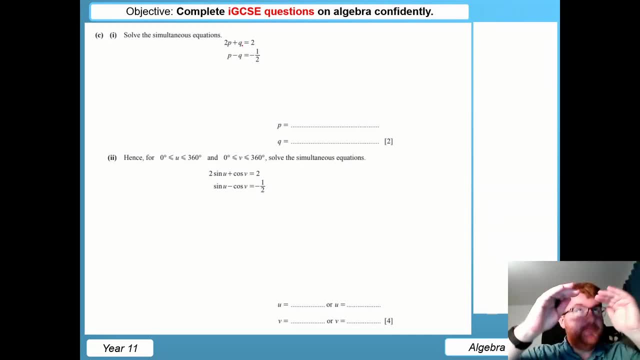 So when we have simultaneous equations in elimination format, what we want to do is eliminate one of the variables. Now, because we have a plus Q and a minus Q, because they're different, we're going to add the two equations together. Have faith, it's going to make the 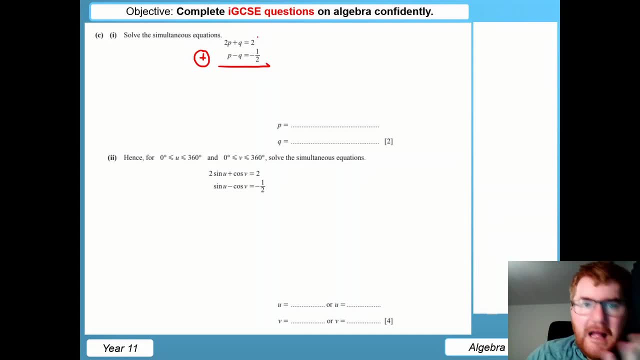 equation work and work out P. Now, if we add them together, what happens? Well, 2P plus P is equal to 3P. Q plus minus Q, that's just zero, which is really, really helpful. And then 2 plus minus a half. 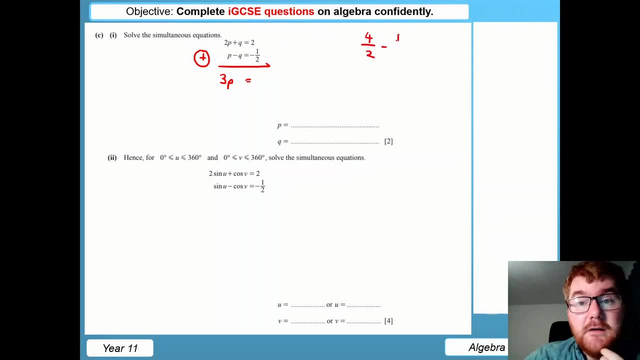 Well, if we do 2 minus a half, that's the same as 4 over 2 minus a half, which is equal to 3 over 2.. So again, I always like keeping things in fractions. You've probably noticed in this video. 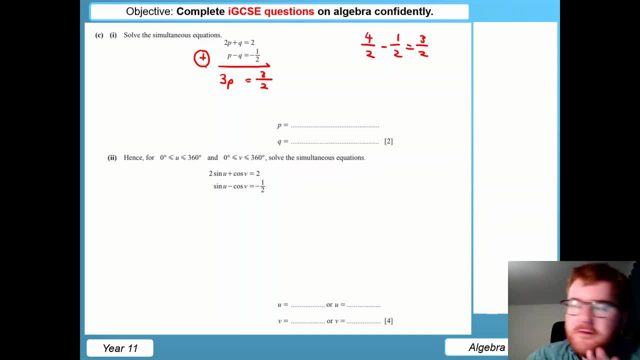 So do keep that in mind. At this point we can do a little bit of jiggery-pokery, as I like to call it. So I want to get rid of the fraction Here. it's another times by 2 on both sides. 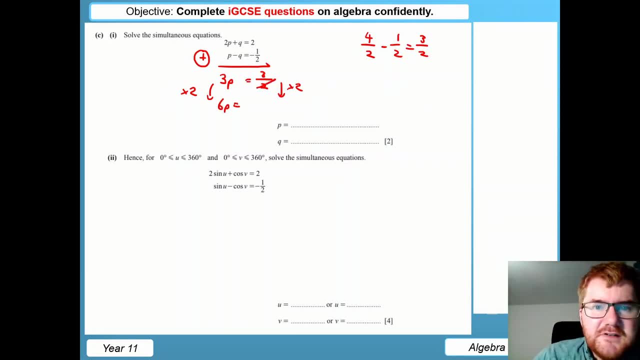 That gives me 3 times 2 is equal to 6P. This cancels giving me 3. And that means that P is equal to 3 over 6, or a half, And it's important to leave it as a fraction. 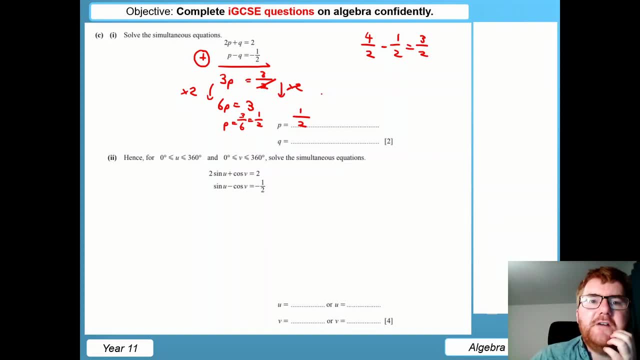 You'll see that for part 2 here. So P is equal to a half or 0.5.. At this point I substitute it back into one of these equations. I'm going to sub in 2, and you'll see why shortly. 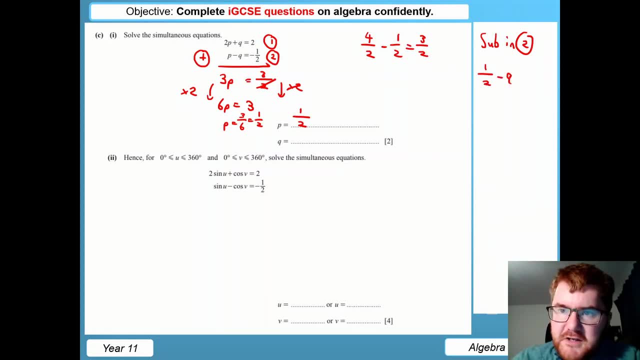 So P is equal to a half, So we get a half Minus Q is equal to minus a half. So I'm going to minus a half from both sides, trying to get that Q on its own. It's a tricky one though. 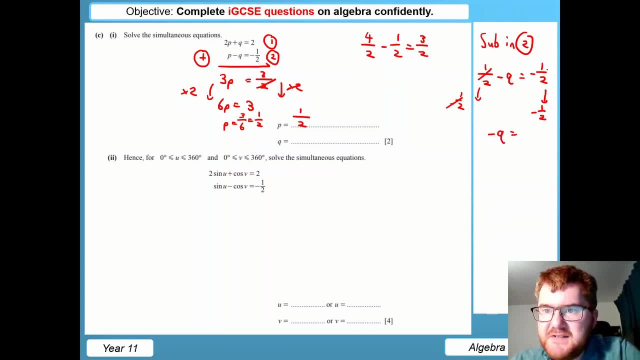 This cancels giving us minus Q And minus a half. minus a half- be careful here- is equal to minus 1. And therefore Q then itself must be equal to 1.. So a fairly standard simultaneous equation question. We saw a quadratic right at the start of the video. 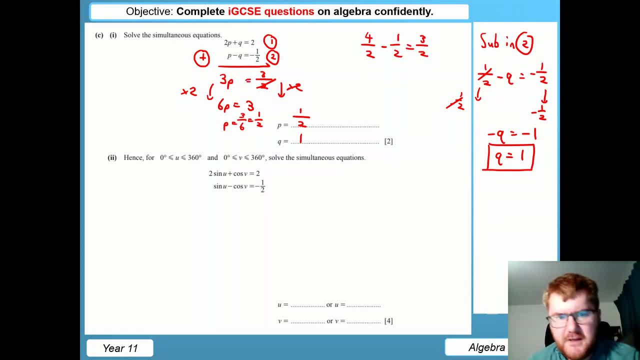 But what the ones to leads to is what's really really tricky here. So hence for the domain of 0 to 360, both for U and V. here we need to solve this equation And again, it's a very similar idea to what we did in part B. 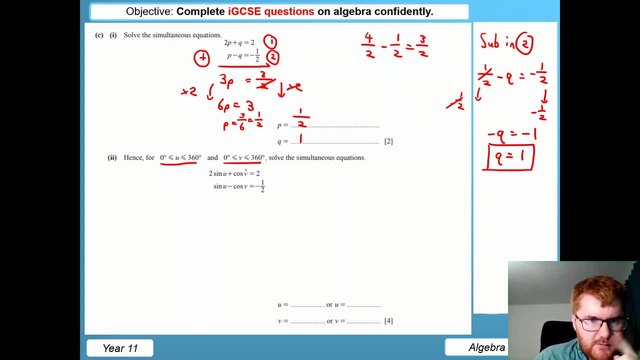 which is? it looks almost identical. Look at the two equations: It looks almost identical. The only difference is that instead of P we've got a sine U And instead of Q we have a cos v. We're not expecting that. 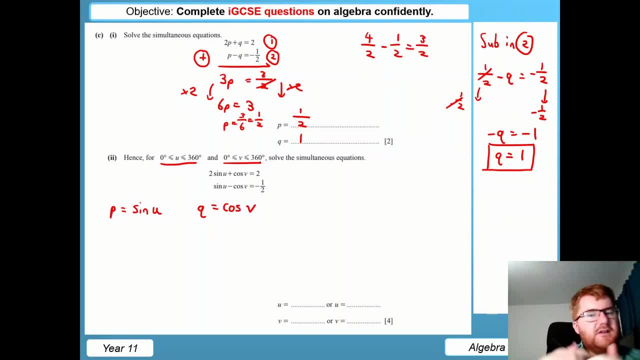 We're hopefully getting this out of home. In fact, there's something we can do. We can write it right back into one in case we're all stuck here. That's kind of thing. to just solve this and use some crazy method. you're trying to use what you've done before. 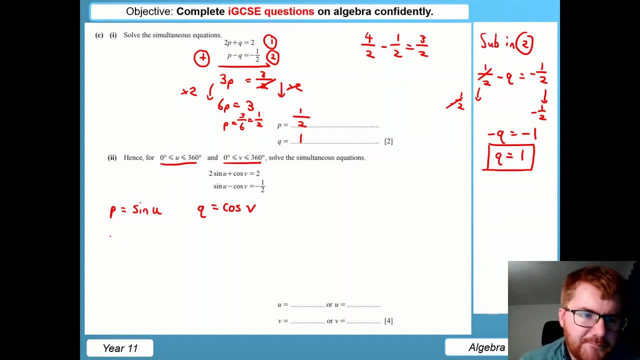 so we now know what p is. p is equal to a half. so therefore sine u is equal to a half, and then cos v is equal to one, and this is where your trig skills really come to the fore. if you need practice on this next topic, then check out the video above. i go through a lot of trig equations where i use 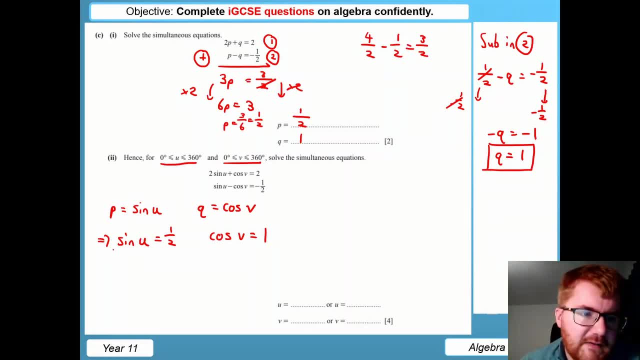 the same ideas as i do just here. now, the easiest way that we do this is: well, we know the sign is. so what's the opposite of sine? well, that's inverse sine on both sides. so that cancels leaving us. u is equal to sine inverse of one over two. now, this is where you can't get lazy with this. 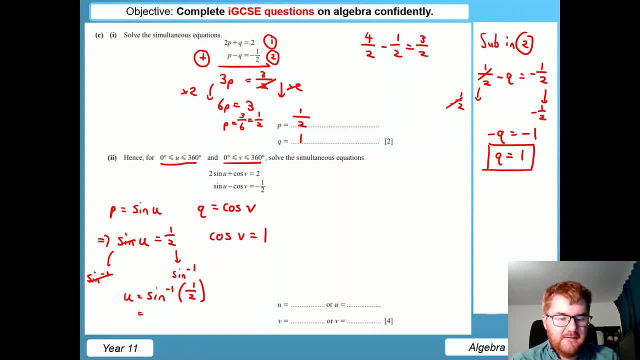 kind of question. so if you do this on the calculator, sine inverse 0.5, you can get the same end of the sign. so on both sides of the equation and on the omdat it's equal to sine inverse is equal to sine inverse of one over two. this is where you can't make its. 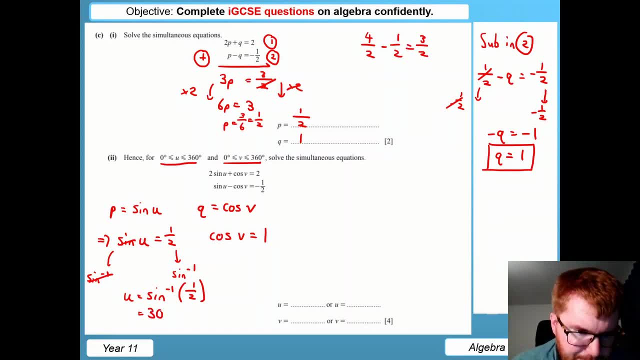 you'll get the value of 30, but notice 30 degrees, but notice there are two values. so use the question here: two values for you and you're probably thinking: where does that value come from? well, let's think about what the sine graph looks like. so the sine graph, it goes. 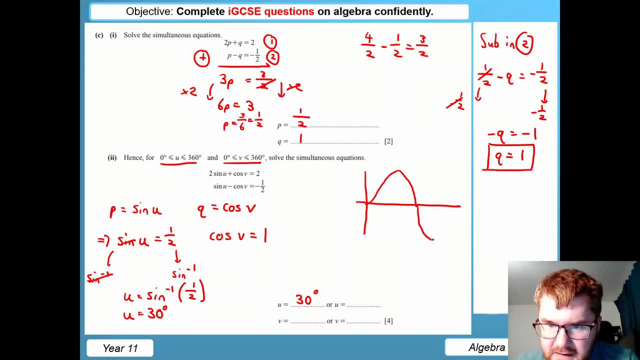 up like this and then down and then down and then like this, so you need to know this off by heart. it's a really important skill also later on in your mathematical career, and the peak here is at 90. I think that's all we need for this particular question and notice. 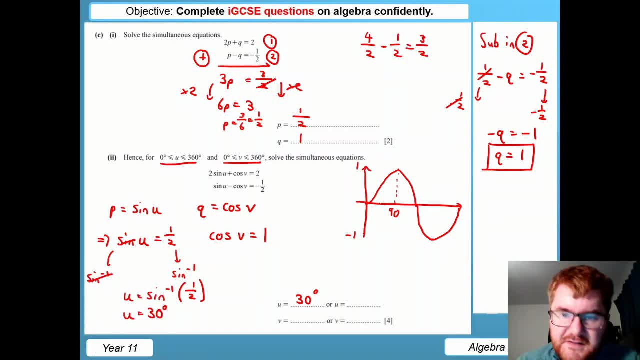 we've worked out. our calculator has worked out one of the answers for us. it's worked out this one, so 0.5 and 30. however, there is another answer over on this side which we have to take into account now. these black lines are the same. notice that middle point. 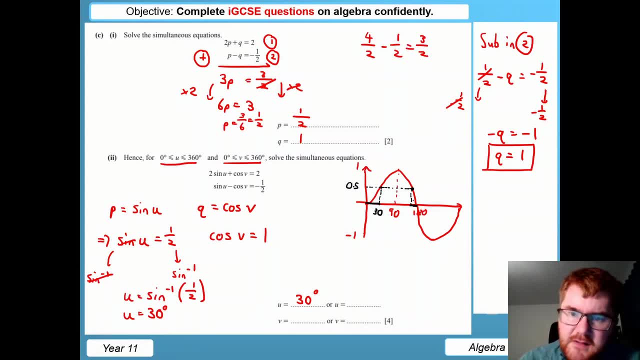 there is equal to 180. So we also need to to get the other answer: do 180 minus 30, which again gives us a hundred and fifty degrees again. I really do encourage you to go back a couple of minutes to check out that video I just mentioned, because this makes a lot more sense once you've seen that. 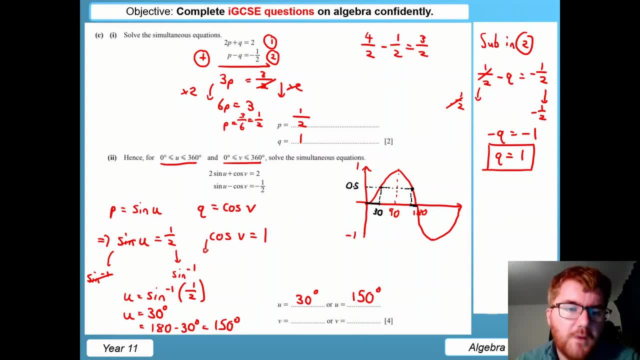 video. now, cos V equals one works in the same way. what's the opposite of co-signing something? we're going to inverse cosine on both sides. this cancels, leaving us just V, and this cancels. this cancels, leaving us just V, and this cancels, leaving us just V, and this cancels leaving. 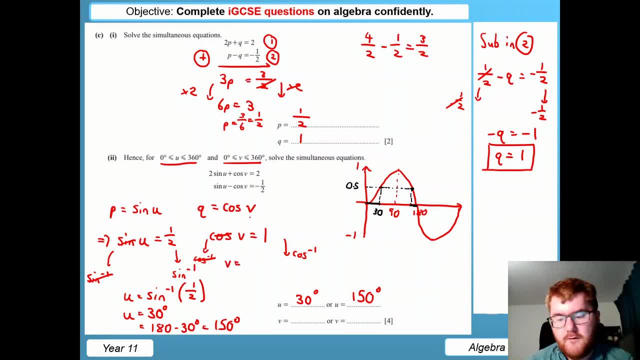 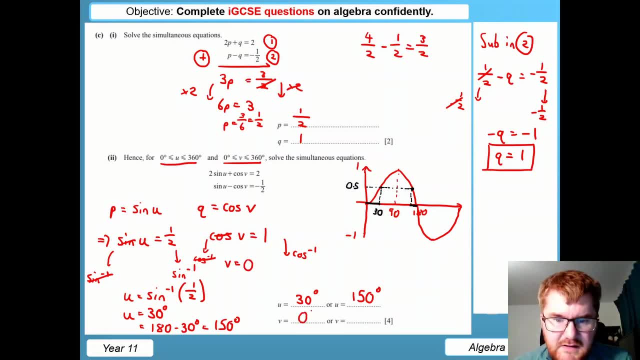 the answer of 0 again. not the only answer here, because if you think of your cosine graph, let me try it on the same one with a different color. it starts at 1, it goes down to 90, down to minus one at 180, comes up at 270 and then goes back to 1, again at 360. so you've got. 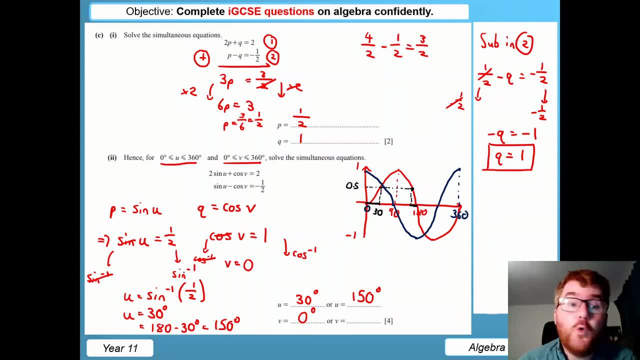 2 answers here: 0, which the calculator works out for you. So we've got two answers here. you can get it smaller, SP for you, cancels, leaving or slightly different, but also the 360 as well. so you need to make sure you put in the 360 degrees, make sure you get all. 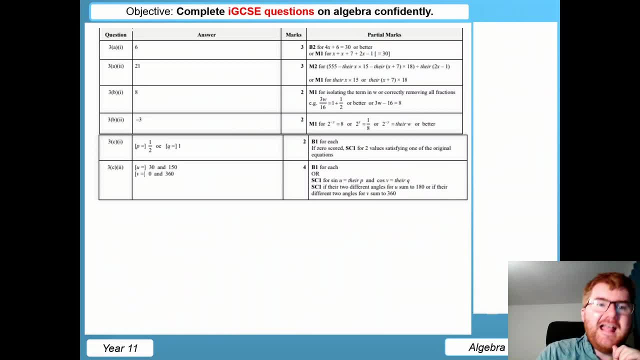 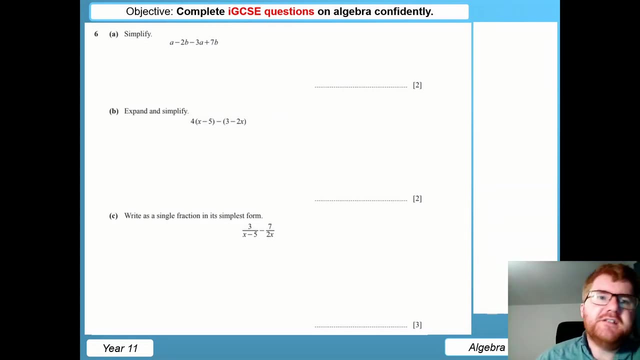 four marks for that particular question and that is the end of that particular question, question 3a, so you can check all the working i've done so far on it. okay, and on to some more typical algebra skills that we haven't looked at so far in the video. so question six here need to simplify. 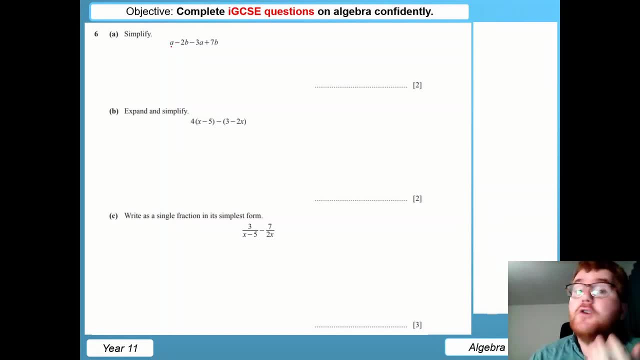 and that means collect those like terms, collect what looks the same. so notice we have a plus a here and a minus 3a which looks the same. so you've got 1a minus 3a. that's going to give us minus 2a- be really careful with negative numbers. and then we've got minus 2b plus 7b. what's that? 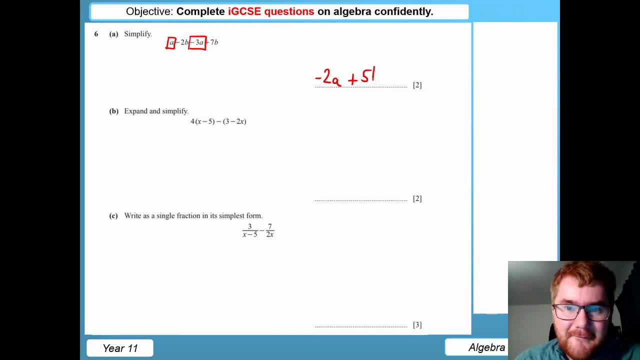 going to be. that's not a pun. that's going to be plus 5b, remember, minus 2 plus 7, plus 7b, equal to plus 5.. And here we're going to do expanding and simplifying- Watch out for these negatives as we go through- And we're going to use what I like to call the hook twice here. So 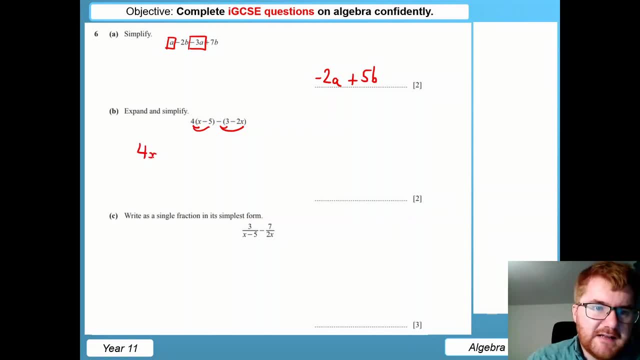 what does that mean? Well, 4 times x is equal to 4x. 4 times minus 5 is equal to minus 20.. This is where the negative comes in here. So minus 1, think of this as a- 1, times 3- is minus 3.. And 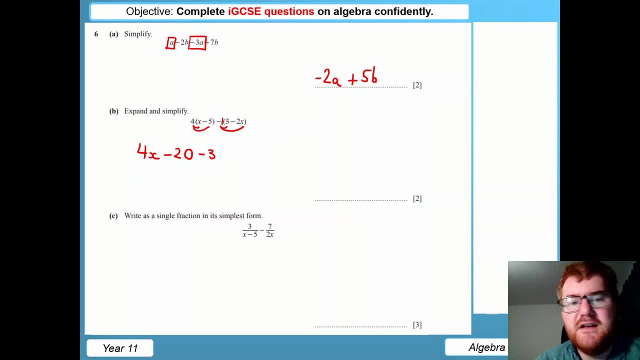 where all students make the mistake is minus 1 times minus 2x is plus 2x. Be careful on that, because now we're going to collect up like terms. So we have 4x plus 2x, that's equal to 6x. 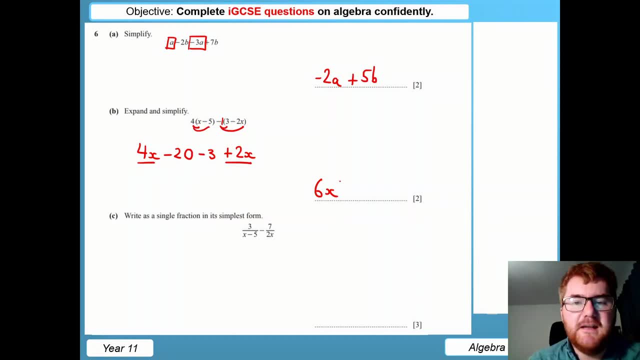 minus 20,, minus 3,- be careful- negative numbers. here is minus 23.. Now, another typical skill is using algebraic fractions, And what we're going to do here is write this as a single fraction in its semantics. So we're going to write this as a single fraction in its semantics. 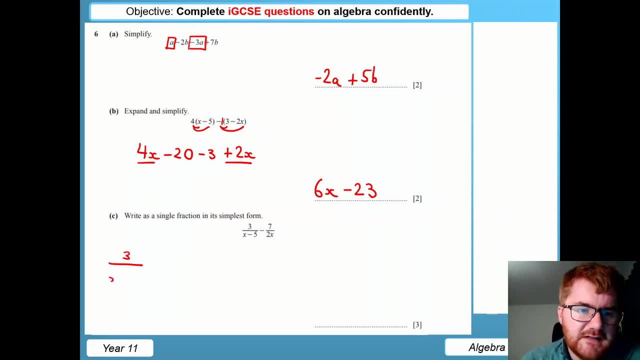 Now the easiest way to generate a common denominator, which is what we need here, is just to multiply the two things together. So on the bottom, we're going to get, on the bottom, 2x times x minus 5.. And to work out the numerators, similar to normal fractions. 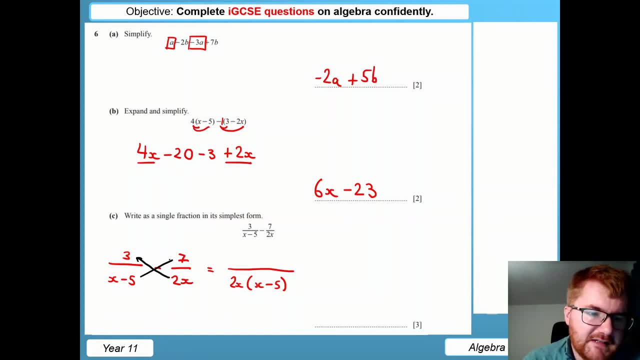 of course, is we're going to times this by this and this by this in order to get the numerator. So, if we do this carefully, so 3 times 2x, 2x is equal to 6x, and then 7 times x minus 5.. Well, we can actually expand this out, So 7 times. 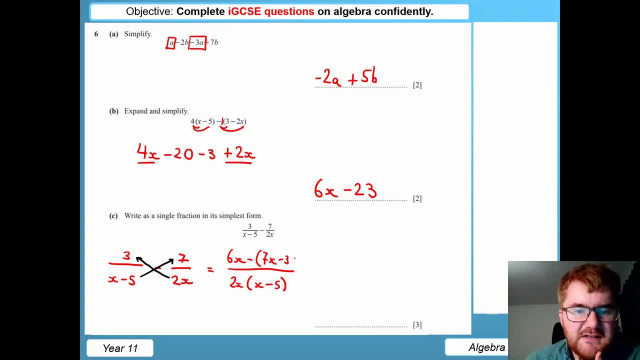 x is 7x, 7 times minus 5 is minus 35. And it wants it simplified in order to check that you know your negative numbers. I've said this before. So if we do this, 6x minus 7x, that's equal to. 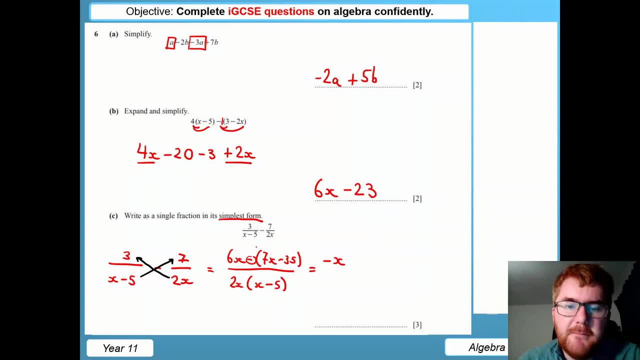 minus x. Notice we've got two minuses here, and the minus and the minus make a plus. We're going to have minus x plus 35, all over 2x open brackets, x minus 5.. Then you can have this: 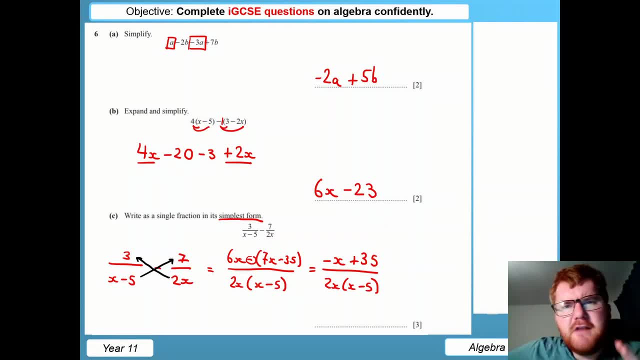 the other way around as well. It's absolutely fine. Just be very, very careful with negatives. It's such a common mistake that's made And through practice you can avoid making those mistakes yourself. And now we're going to solve this equation And hopefully you're getting sort. 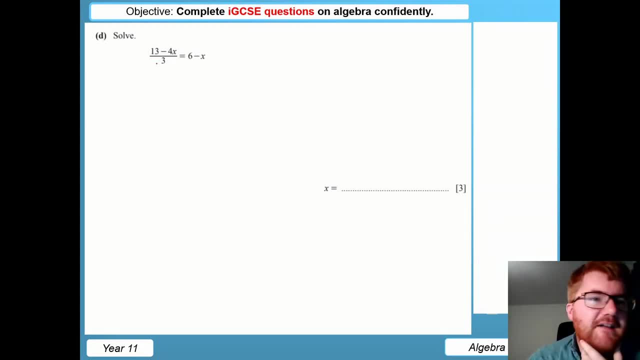 of the patterns of the questions. at this point in the video I see a fraction. I don't like fractions. What's the opposite of dividing by 3?? We're going to times by 3 on both sides. This cancels, giving us something quite nice: 13 minus 4x. And then we times both of these by 3.. So be careful. 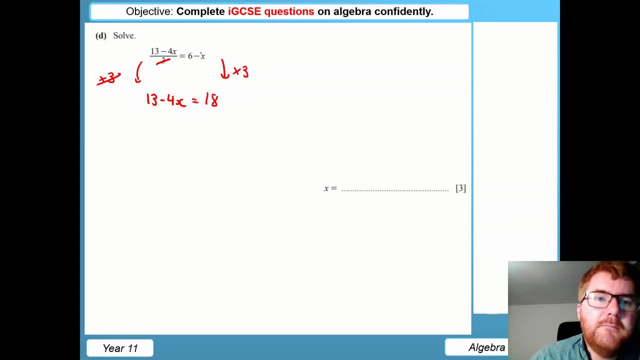 with that. So 6 times 3 is 18.. Minus x times 3 is minus 3x. Now the way to simplify this really really quickly is: look at the fewest amount of x's. So minus 4 is less than minus 3.. And now we 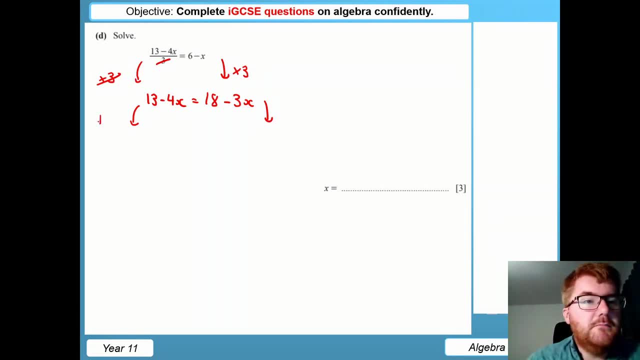 can just work out x. So what's the opposite of minusing 4x? We want to plus 4x on both sides. Watch the magic happen. So we cancel this out. We're left with just 13.. 18 stays as it is, And 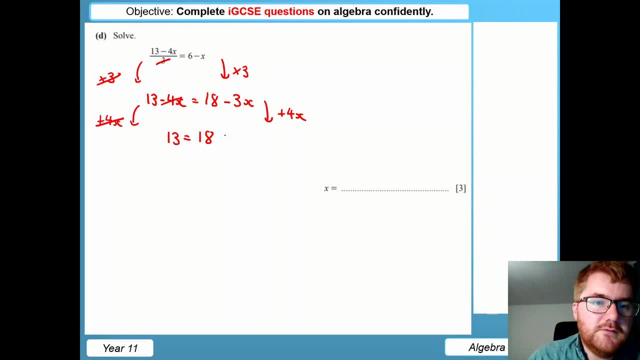 then minus 3x, plus 4x, that's equal to plus x. Notice, a lot of the difficulty disappears after that step. And now we can just work out x, because the opposite of adding 18 is minusing 18 on both sides. So we can just work out x, because the opposite of adding 18 is minusing 18 on both. 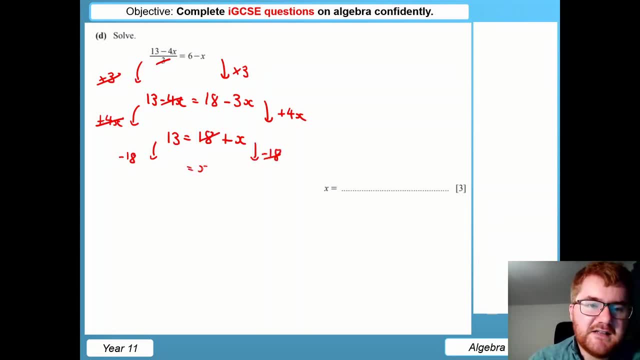 sides. So we can just work out x, because the opposite of adding 18 is minusing 18 on both sides. This cancels, leaving us with just x And then 13 minus 18, checking your calculator, if you're not happy with it, is minus 5.. So we pop that in And there's other parts of the question, because 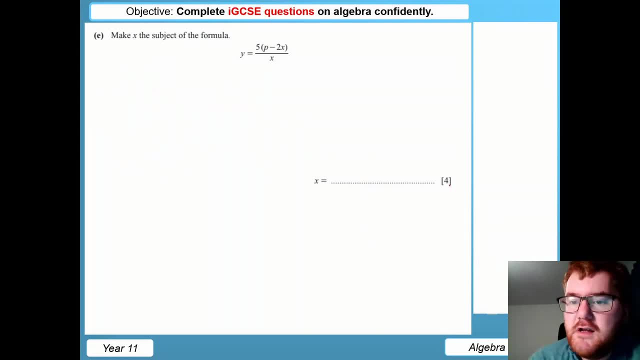 it's a paper 4 question And this is quite tricky. So this is why it's a 4-mark question. Use the amount of marks in the question to really guide how much work you think is going to be in the question. So make x the subject of the formula. So what this means in normal English is that you're 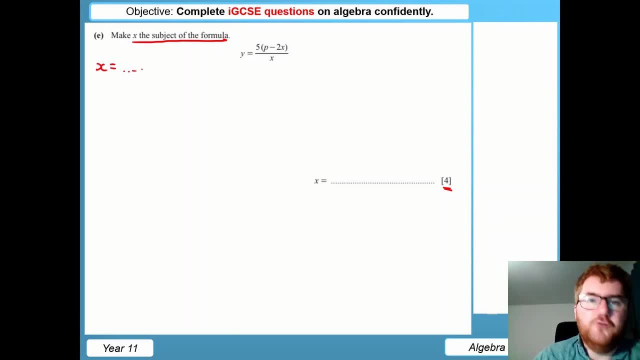 going to want. x equals something in terms of not x, basically, Right. How do we do that? So, first thing is, I don't like fractions. You're probably getting the hang of that by now that I don't like it. So what's the opposite of dividing by x? We're going to times by x on both sides. Well, x times y. 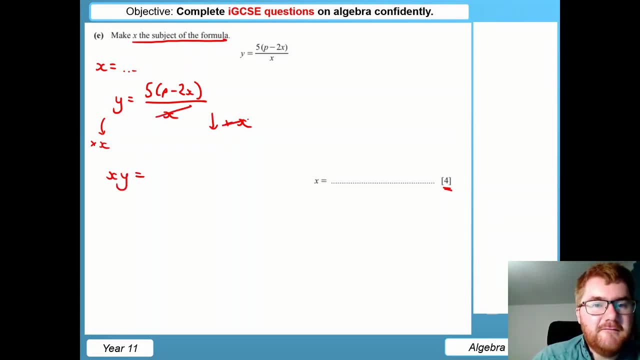 is just xy, This disappears. Fantastic, We get 5 lots of p minus 2x. Now the general strategy with these kind of questions, with lots of xs in the question, is to get everything with x on the left-hand side and everything else on the right-hand side. So you: 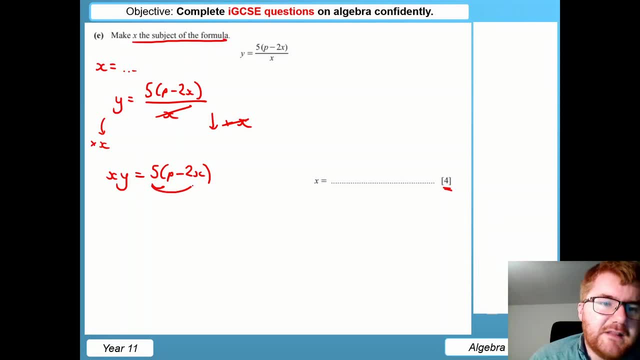 can see that in the next couple of steps here. First of all we're going to expand the bracket using the hook. That then gives us: 5 times: p is 5p, 5 times minus 2x is minus 10x, And following: 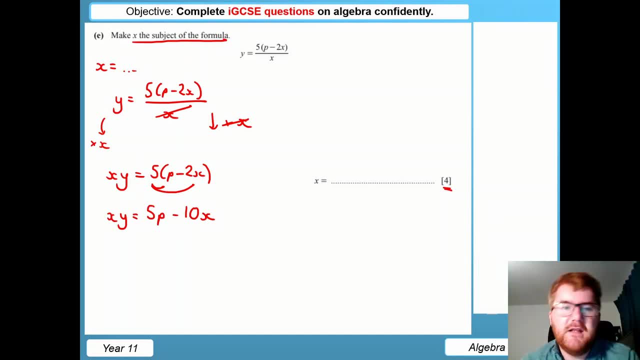 that principle, I'm going to put all the xs on the left-hand side. So what's the opposite of minus 2x? We're going to add 10x on both sides. Feels like we're not making progress, but do bear with. 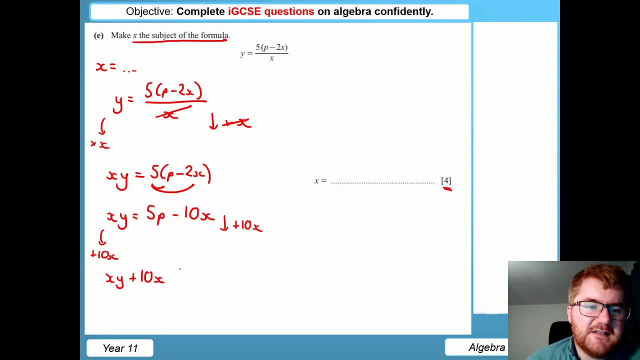 me. So xy plus 10x is equal to well. this cancels, leaving us with just 5p, And this is where the magic is going to happen. So notice, there is a common factor here: They both share an x, So we. 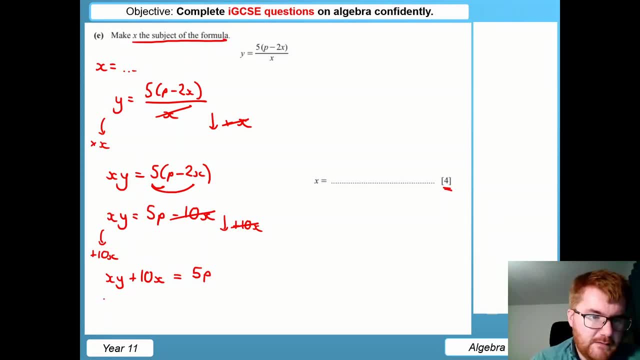 can factorize into a single bracket. So I'm going to set up my bracket ready and now work backwards. So what do I multiply x by to get xy? Well, just y. What do I multiply x by to get 10x plus 10?? And now notice, we've only got one term of x, what we wanted. So 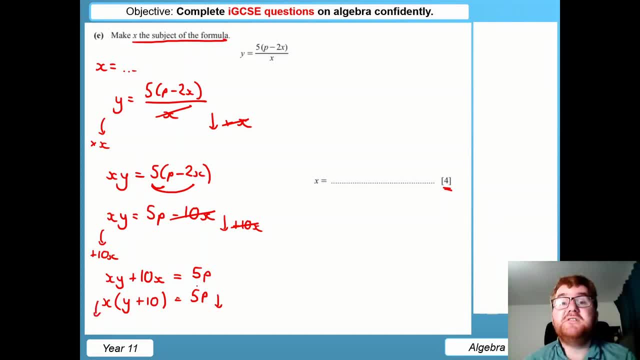 now we need to get rid of that y plus 10.. So what's the opposite of timesing by y plus 10?? Well, dividing by y plus 10 on both sides, So we get 5p over y plus 10, giving us all four marks. And when we get quicker at these questions, 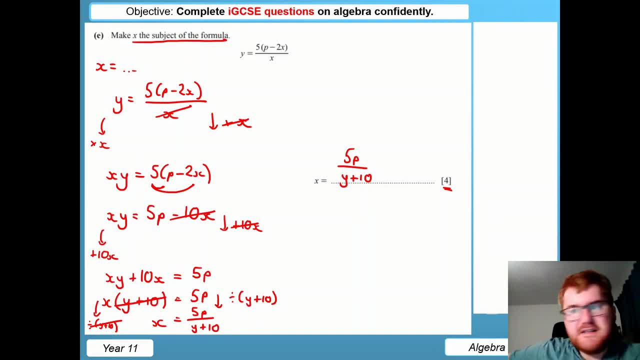 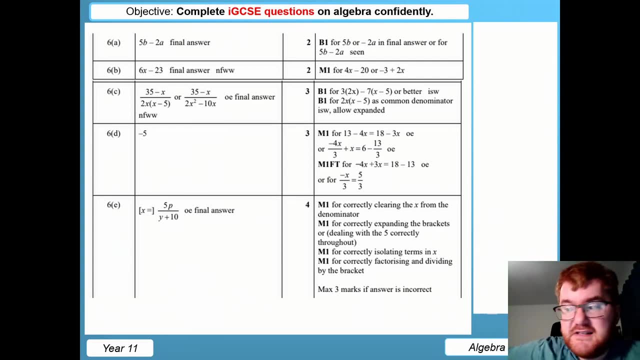 these are quite an easy four marks to get Definitely the A-grade end of the spectrum, but very, very achievable. All right, so you can check all the answers that I've gone through in question 6e so far, And now let's move on to some factorizing. If you found this video, 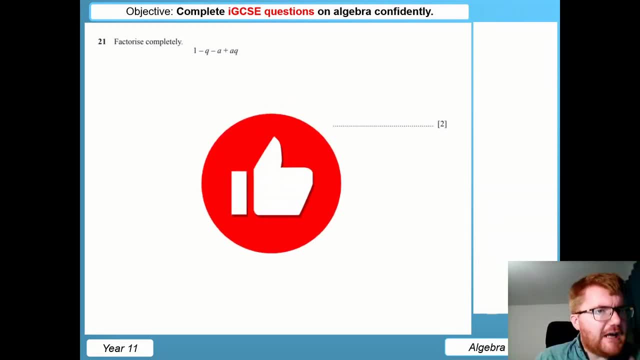 really useful for you. subscribe to my channel and I'll see you in the next video. All right, so if you've enjoyed this video so far, then please do subscribe to the channel, because I'm bringing out lots of IGCSE videos, really trying to fill in those gaps for you. 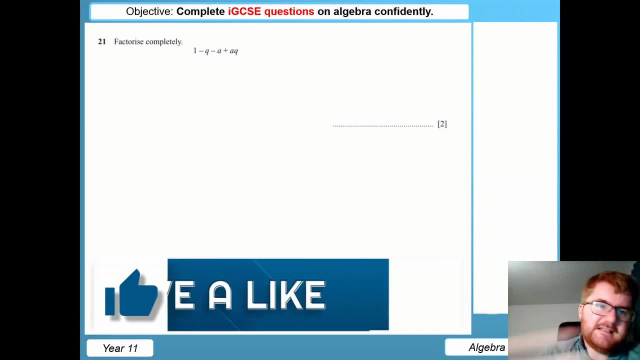 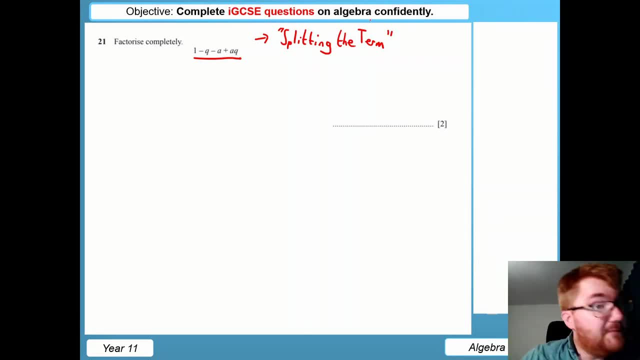 this is the last step of splitting the term. if you do this, If you're not familiar with that term, that's absolutely fine. I go through this from basics. So what I'm going to do is I'm going to separate this down the middle, like. so. You're thinking: what am I up to here? Well, let's have. 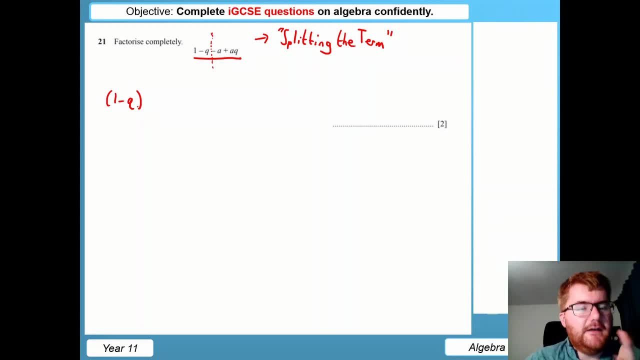 a look. So we've got 1 minus q, left-hand side of that line, And then we've got minus a plus aq. Notice we can factorize that There is a common factor of a. So I'm going to take out. 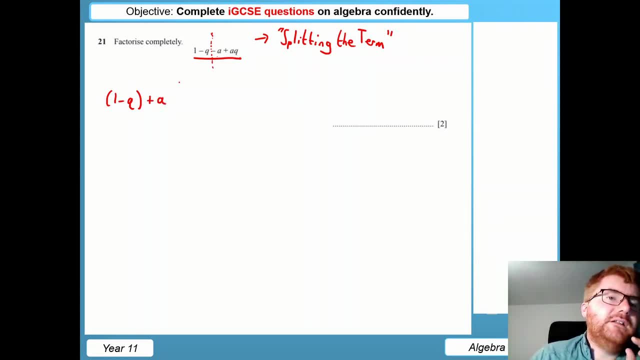 a factor of a. Now notice, I take a factor of plus a out, So you'll see that in a moment. What do we multiply a by to get minus a? Well, we get minus 1.. What do you multiply a by to get aq? 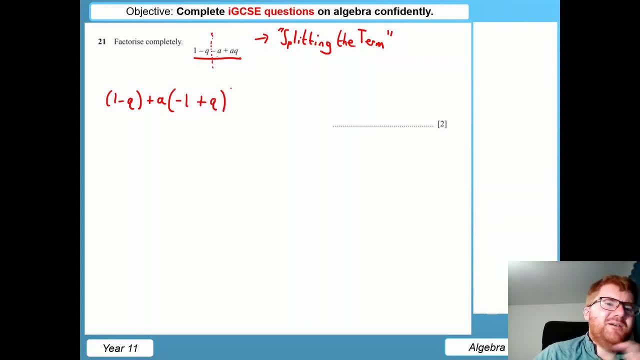 plus q. And you look at this and go: ah, it's almost the same in both brackets, but not quite. And the way that we can change this- so I want to make that mistake on purpose- is if we change this to a minus. 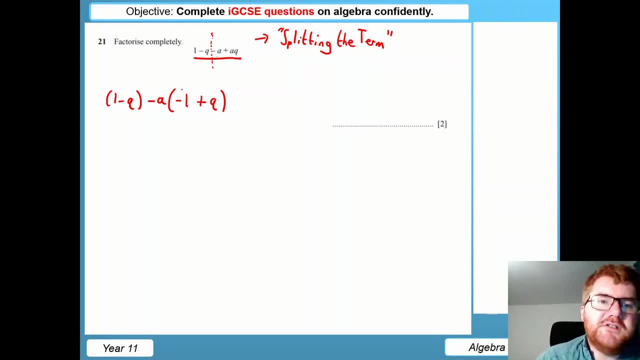 then we can just switch the signs and we get exactly what we want in the bracket. Again, if you're not sure about what I'm doing at this particular point, then let's just go backwards. If you do minus a times 1, that's minus a, That's all good. Minus a times minus q is plus aq. 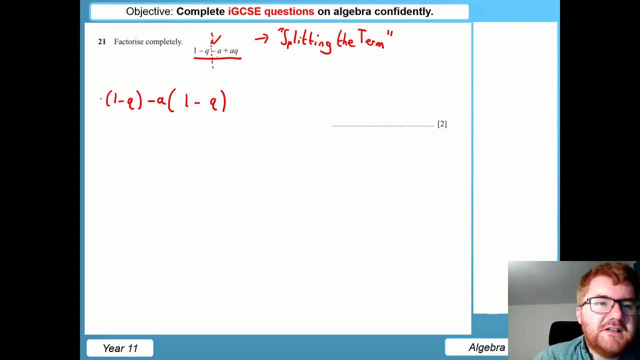 So I've just put this into a single bracket And now the magic is going to happen at this point. Now I've put a 1 out here, just so you can see what's going on. If we look at this expression, what do they have in common? Well, they have a 1 minus q in common. 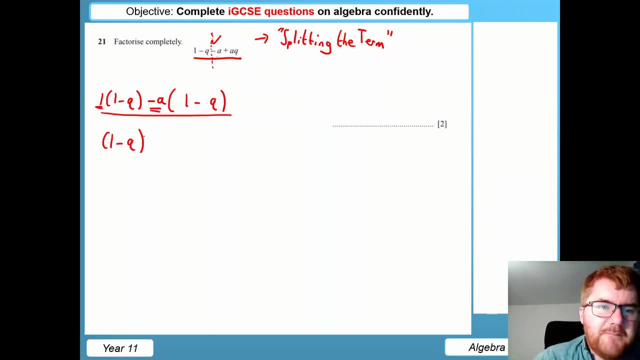 What's left outside? Well, we have a 1 here and a minus a. We put that into a second bracket, So we get our final answer of 1 minus q, 1 minus a. Now, if that seems like complete wizardry to you, that's absolutely fine. 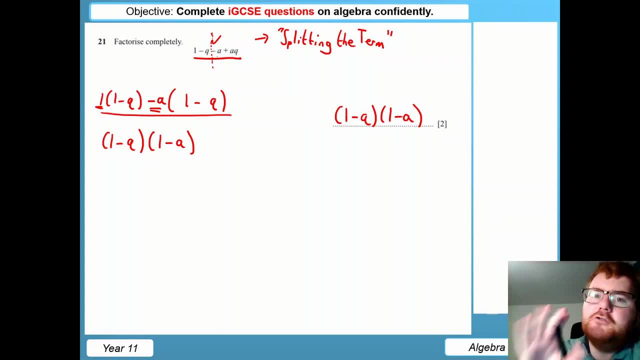 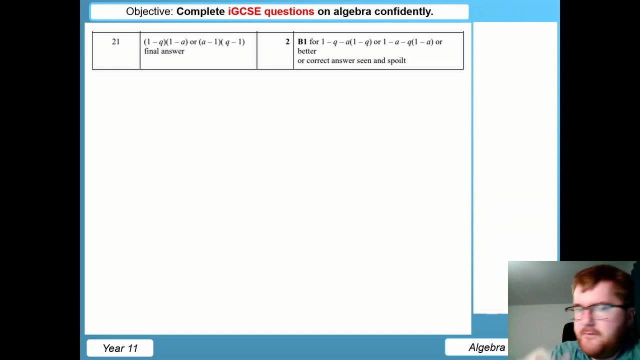 If you see this technique more and more, it gets easier. But if you're not sure of that answer, expand it and see if you get back to the original question. So there's the answer. So there again, you can have it both ways round as well. 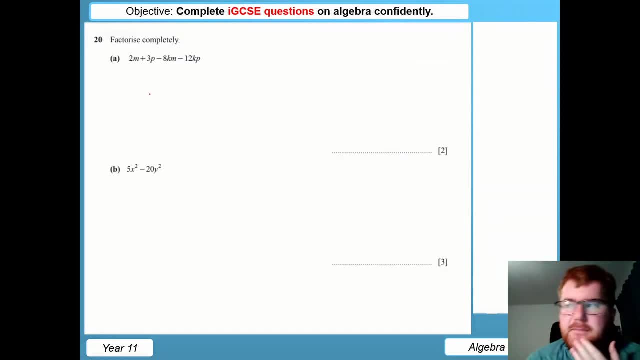 And I want to continue showing you questions like this. So again, similar idea. at this point We've got 2m plus 3p, minus 8km, minus 12kp. This kind of question comes up quite often. Again, I'm going to split this down the middle. 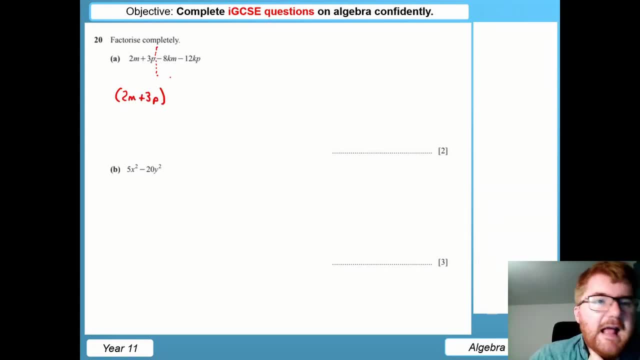 So we've got our 2m plus 3p, And now I'm going to take a factor out here. I'm going to take out a factor of: well, they have a 4 in common, a minus 4 in common. 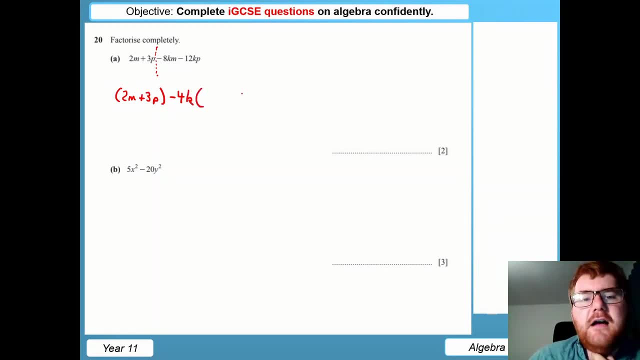 And they also have a k in common. So I'm going to take that out. And now I'm going to work backwards. So what do I multiply minus 4k by to get minus 8km? Well, I get minus 2m. 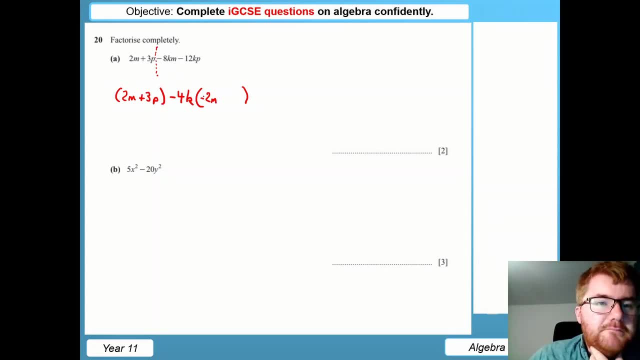 What do I multiply plus 2m? There we are. And what do you multiply minus 4k by to get minus 12kp? Well, 3p Again, we achieved what we wanted to achieve here, which is that the 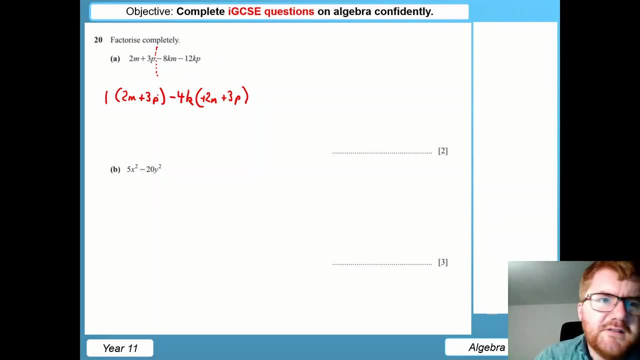 the brackets are exactly the same. So at this point we take out the common factor of the bracket, So 2m plus 3p and whatever's left outside. So we've got a 1 here and a minus 4k that goes in the second bracket. 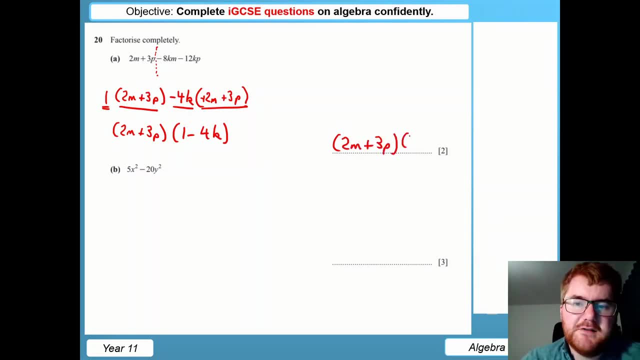 Again. I'll pop the answer over here for you as well. Perfect Again. expand it if you're not sure. that gets to the same answer as you see in 28.. Now, 20p is a kind of different style of question. 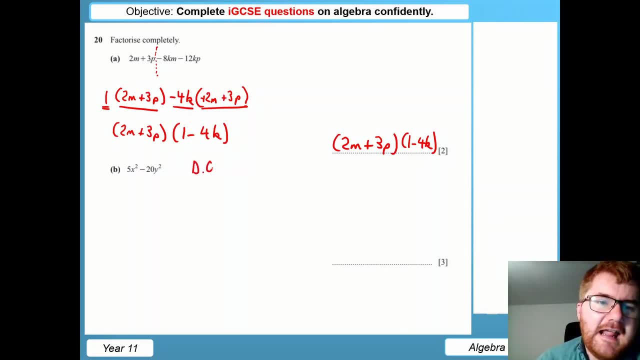 Here it's going to be something called dots, which I'll be explaining in a moment. The first thing, as I always do in looking at these questions is: is there a common factor? There is, Five goes into both, So I'm going to take a factor of five out here. 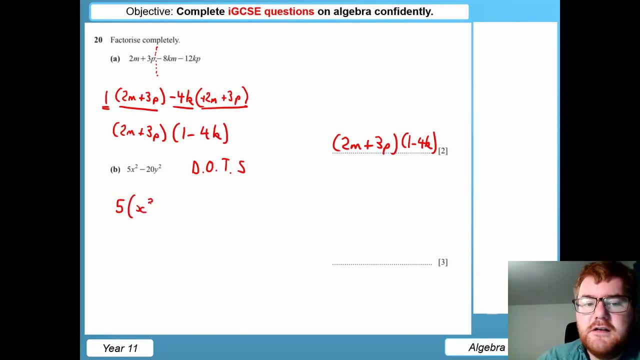 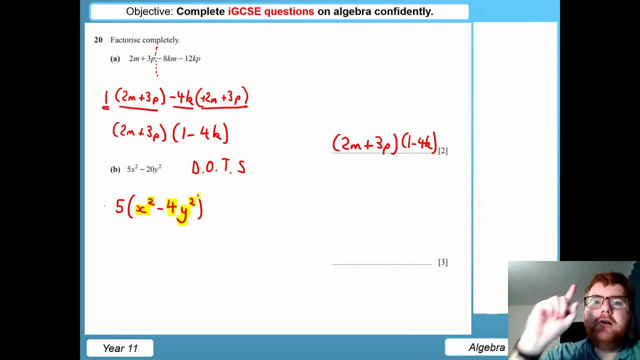 And we have a y squared Bells should be ringing in your brain at this point. If you have all square numbers in a bracket. we want to use the idea of difference of two squares: D-O-T-S. Now what does that actually mean? 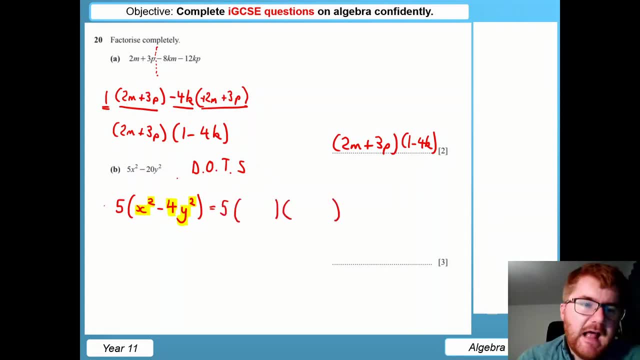 Well, it means we can put it into two brackets and we take the square root of each number. So the square root of x squared is x. Square root of 4 is 2.. And the square root of y squared is y, And we put that into both brackets. 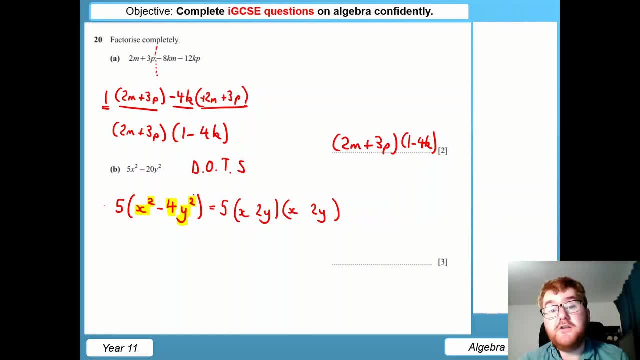 And in order to remove the cross terms. so when you multiply the brackets we make one plus and one minus, And this is a technique really to recognise more than anything else and just practise at home So you can answer those kind of questions and get all three marks. 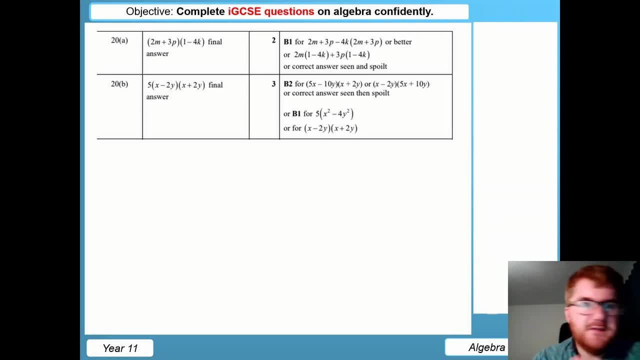 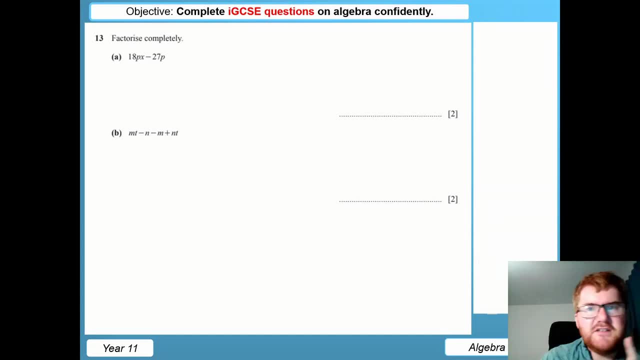 So you can see the answers there. So make sure you go through that nice and carefully. And yes, we've got some more factorisation, because I'm imagining at this point of the video you're still a little bit unsure with this weird factorisation. 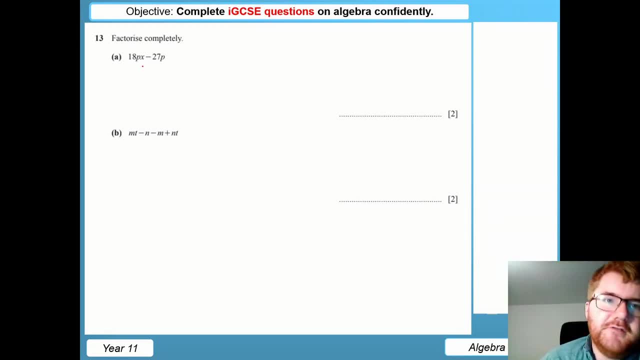 No problem, I'm here to help you. So let's go through this again. We look for common factors, So we notice we've got 18 and 27.. Well, 9 goes into both and a p goes into both. And now we work backwards. 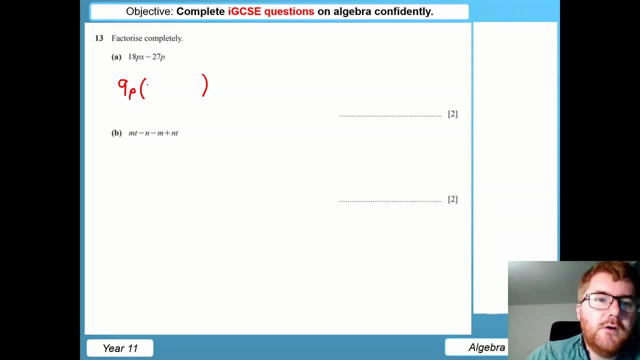 So what do we multiply 9p by? to get 18px? Well, 2 and x. What do we multiply 9p by? We multiply to get minus 27p or minus and a 3.. So notice all the different varieties of different factorising questions they can give you. 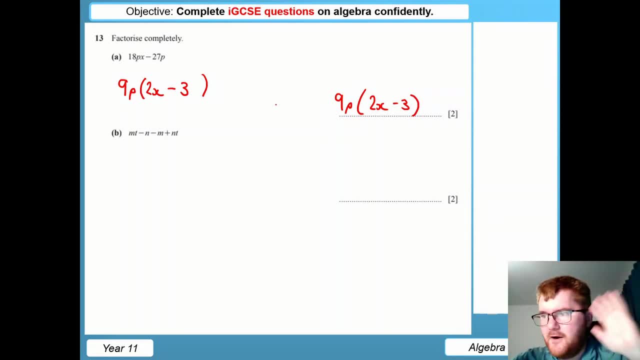 And if you look at question B, hopefully your alarm bells are going off. It's one of those. There are four terms. They all look kind of similar as well. We need to divide it down the middle, So it's one of those kinds of questions. 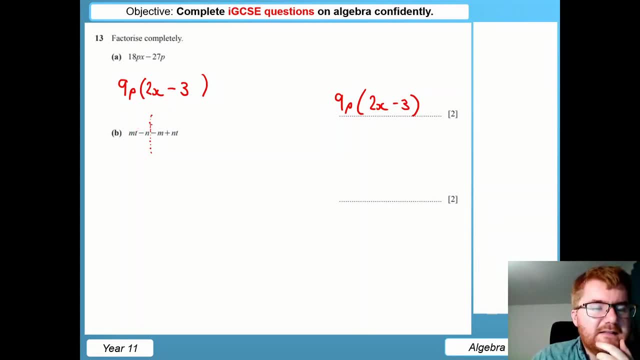 However, if we try and factorise here down the middle notice, there isn't a common factor. So this is an even harder question than what we looked at before. So what I'm going to do is I'm going to move this around slightly. 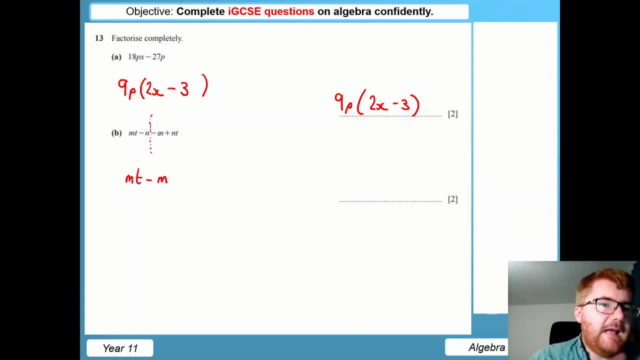 I'm going to put an mt minus m. So I'm going to bring the m's together, And then I'm going to put a plus nt, minus n. So I'm putting the m's together here and I'm putting the n's together. 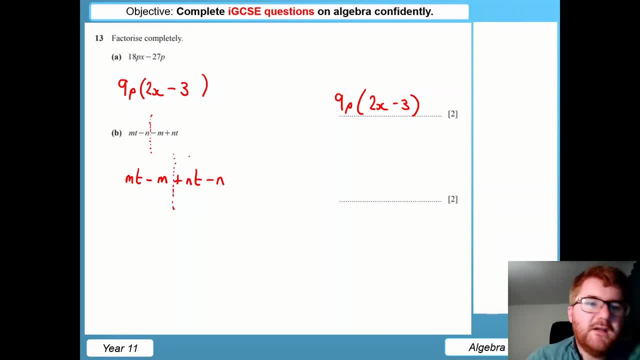 And now there's a common factor. When I draw this line down the middle, I can factorise both of them into single brackets. So let's look at the left hand side. They both have an m in common, And what do we multiply? 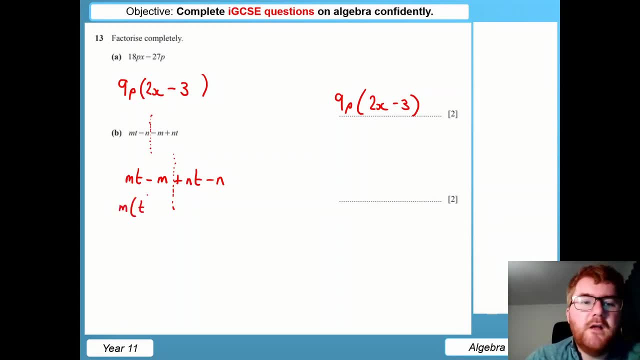 And what do we multiply m by to get mt or just t? What do you multiply m by to get minus m Minus one, And we get exactly the same on the other side. So I have an n as a common factor. What do we multiply m by to get nt or t? 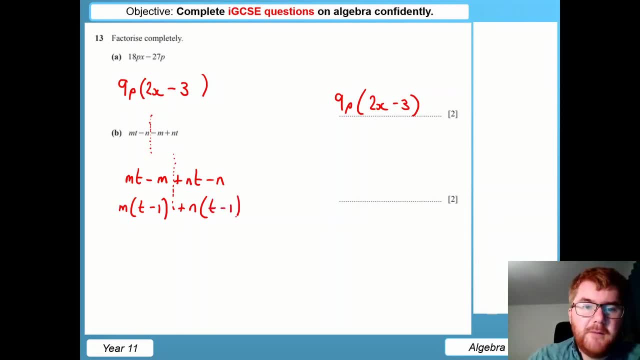 What do you multiply m by to get minus n? Well, minus one. Notice, by moving around the terms, which is quite sneaky here we actually get that form that we're quite used to from previous questions. Notice, they have a t minus one as a common factor. 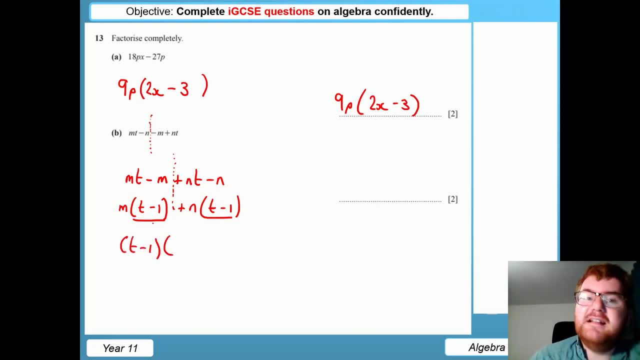 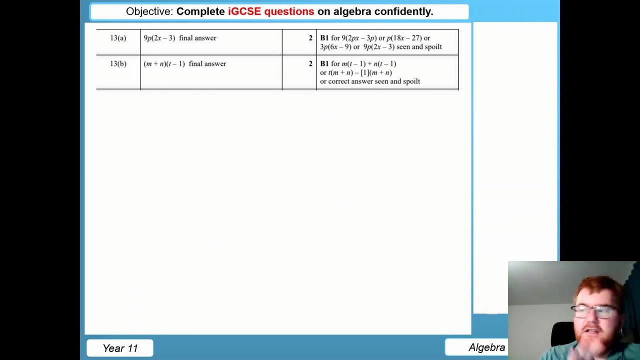 So we put that as our first bracket. Anything left over, well, m and n go into our second bracket. So we get the answer of t minus one and m plus n Super-duper, And you can check the answers very quickly there. 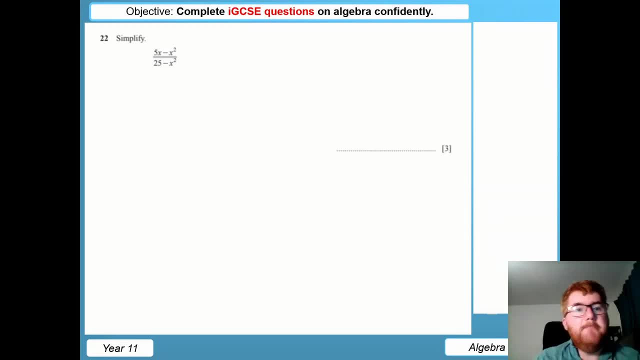 And let's look at again a slightly different style of question, mixing what we've done with factorising, but also algebraic fractions as well. So they want us to simplify this particular expression. So the first thing that comes to mind here is: well, can I factorise? 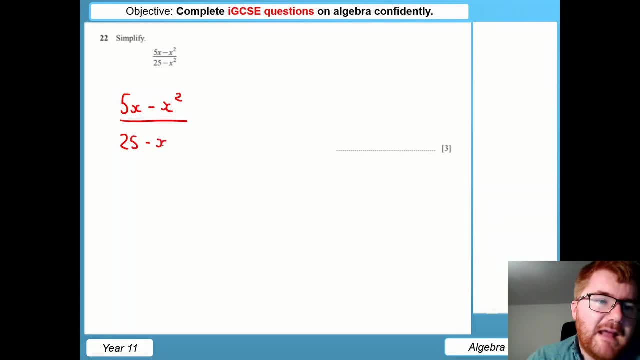 That's what I'm always looking at. Can I factorise? Maybe that will help. Well, the top is probably the straightforwardest here, because they have an x in common. So let's take a factor of x out. What do you multiply x by to get 5x? 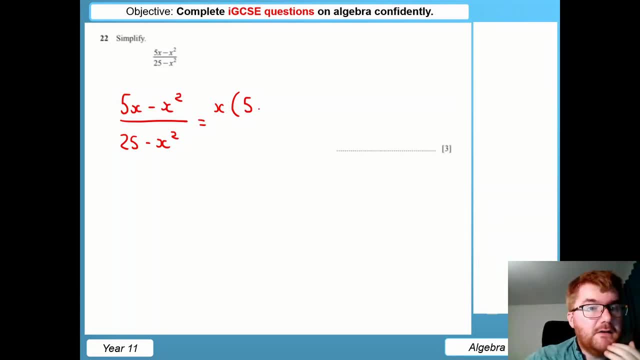 Well, 5. What do you multiply x by to get minus x squared? Well, minus x. OK, that's interesting. And now the bottom is ding, ding, ding, ding, ding. One of those. you've got square numbers. 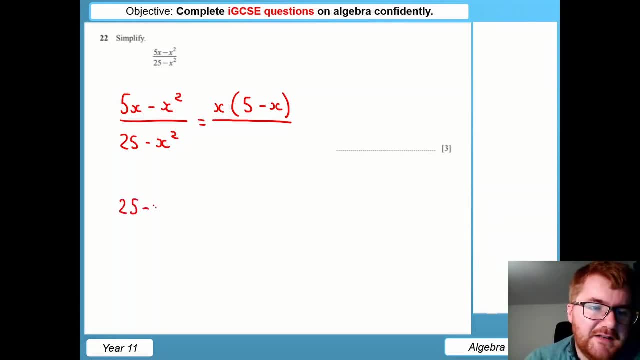 So if we take 25 minus x squared, we can set up the two brackets And notice we can take the square root of everything. So the square root of 25 is 5.. The square root of x squared is x And because we want the cross terms to cancel, we put a minus in one and a plus in other. 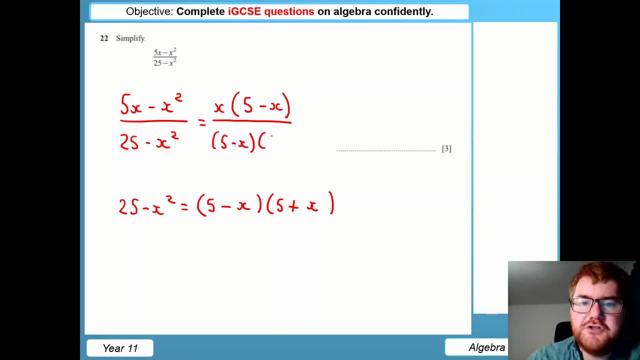 And you really need to spot this on the higher-level questions. Now, what's the whole point of doing this process? It's easy. We've got a common factor here. Well, you'll see, here we've got a common factor top and bottom, so we can cancel. 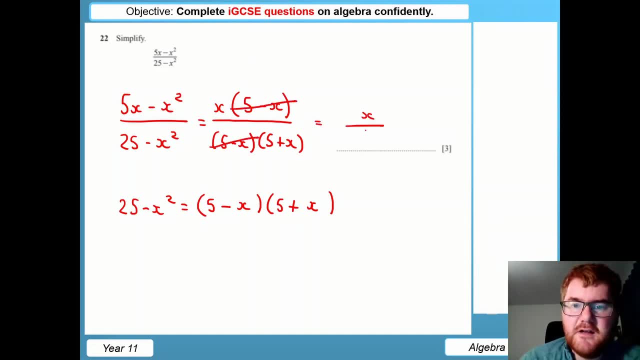 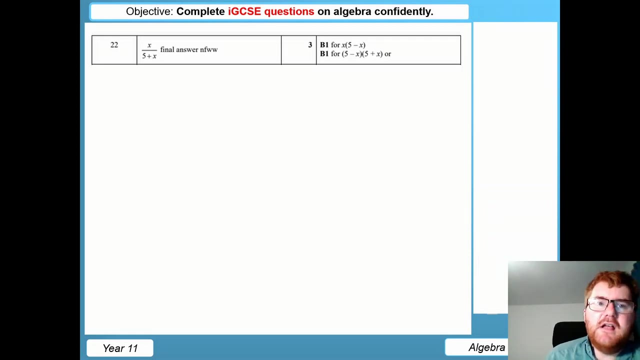 And we're left with our final answer here of x over 5 plus x. When you see these questions and you know these questions, these are nice, easy three marks to get with a bit of practice. OK, so you can see that you get the final answer there of x over 5 plus x.